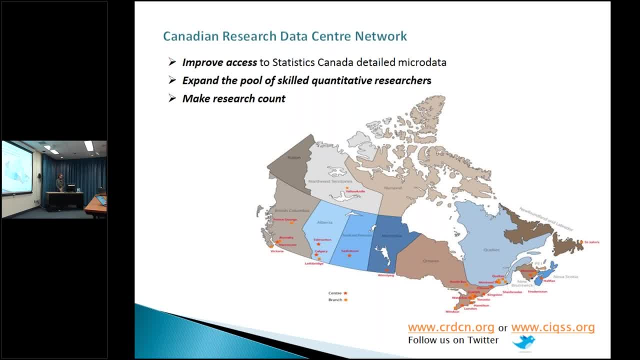 These facilities are secure computer labs where researchers with an approved project can access Statistics Canada, confidential microdata from a variety of surveys, including the longitudinal surveys, census data, of course, and an increasing number of administrative data sets. Last year, more than 1,500 researchers from various 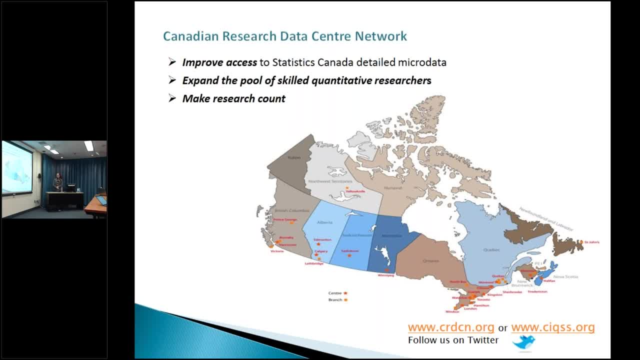 disciplines have access to an RDC across the country and about a third of these were graduate students. The research they carry through the network is very diverse and help to better understand social economic developments affecting the whole society as well as factor affecting individual life course and 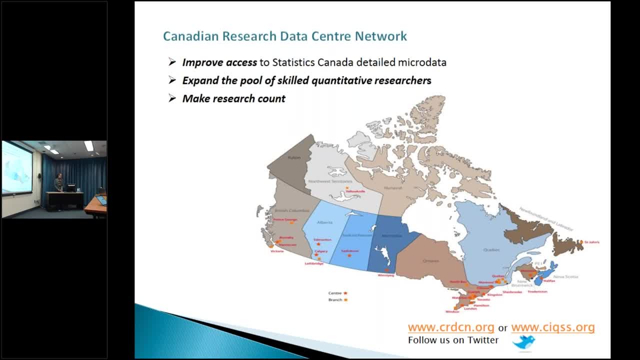 well-being. This includes, among other topic, population aging, economic integration of immigrants, socio-economic determinants of health, income and equality, labor market participation and child development and soon, we hope, business dynamics. So to know more about us, I invite you to visit our website you. 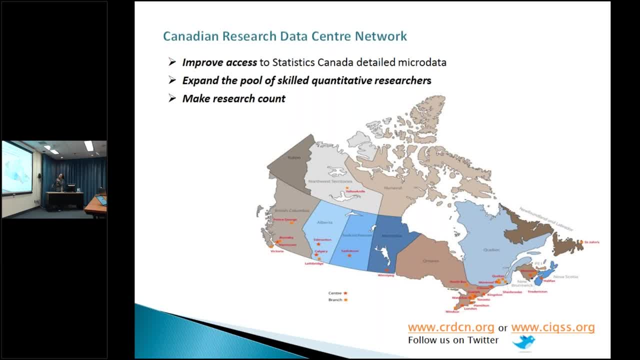 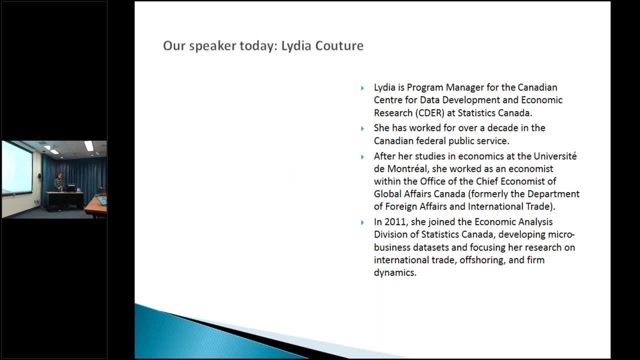 see the the address on the slide, as well asitolieskicks if for those of you who would like to know more about the SICK as well. So, without further adieu, let me introduce our speaker for today. Ly serpent is been working for the Canadian Federal Public Service for Brenda 2013,. Lpected Public Programme as BLT城ü stamina. Recreation No 0 nine: personal knowledge about苦stan. further ado, let me introduce our speaker for today, Lydia is. he's been working for the Canadian Federal public service for. 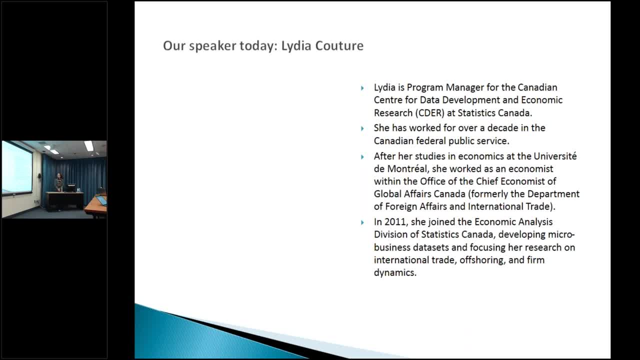 over 115 129 10ster. Salute to coming from Canada, the decade now. she is currently program manager for the canadian center for data development and economic research, the cedar, at statistics canada. she's previously worked as an economist within the office of the chief economist of global affairs canada and in 2011 she joined the. 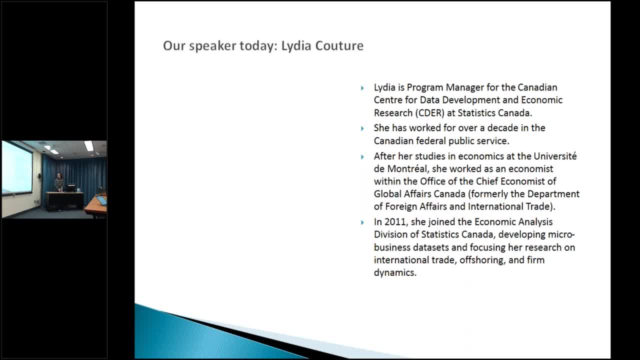 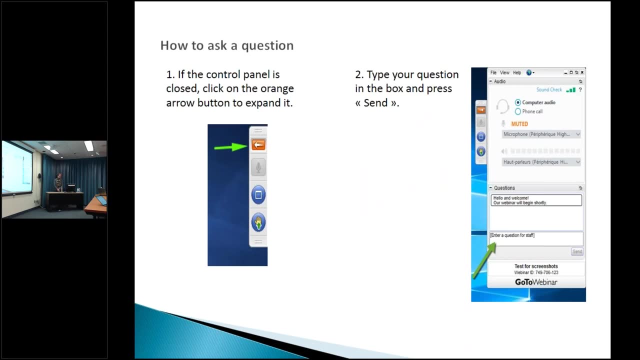 economic analysis division at statcam where she contributed at developing micro business data sets, and she's mostly interested in international trade, offshore offshoring and firm dynamics. so lydia will speak for about 40- 40 minutes and then we'll have a q a period. i invite you to write. 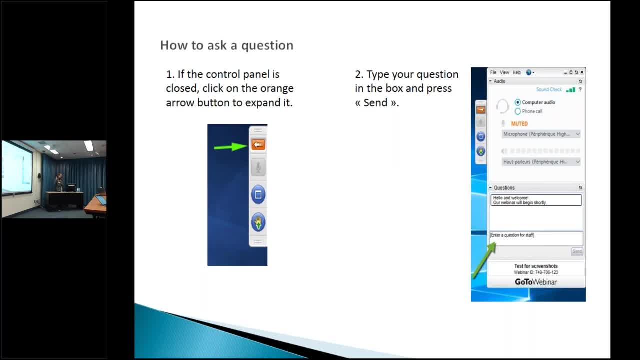 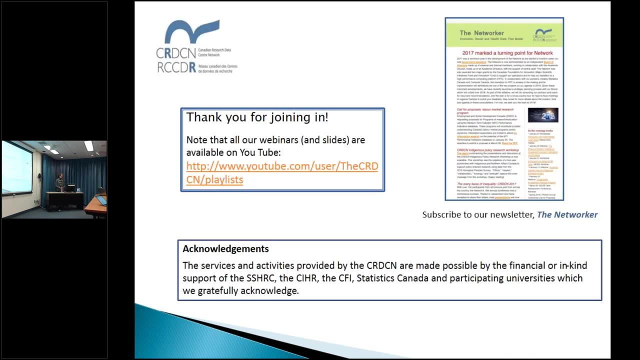 down your question by opening your control panel. you will see there's a section where you can write questions. so i will read them after her presentation for you and she will then answer them. so thank you again for joining us. um, um, just wanted to mention that, uh, for your colleagues. 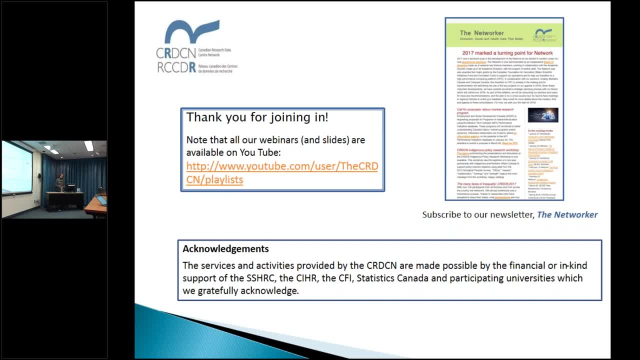 or for yourself. if you would like to revisit the webinar, it will be available on youtube afterwards. um, give us a couple of days. it should be there. um, after easter. let's say all right, so that's it for me. thank you again, lydia, for joining us. uh, the mic is now over to you. 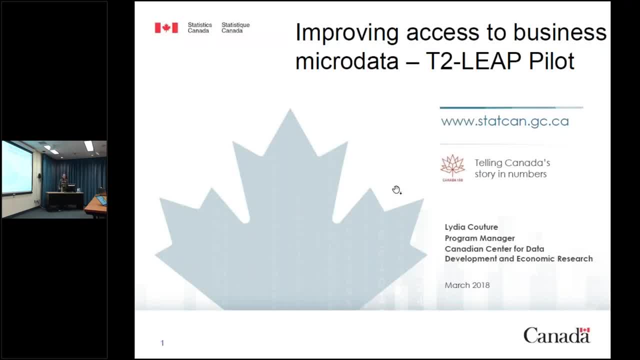 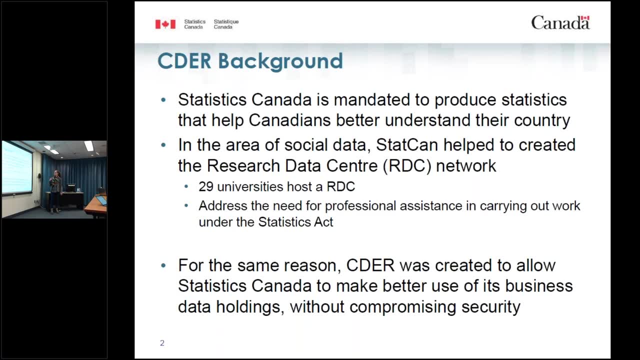 um, all right, thank you very much for having me today. um so, cedar, so what do we do? uh, so, i think people are familiar with the research data center network and the research data center and what they do, as you might know: statistics. canada is mandated to produce statistics that helps canadians better understand their country, the economy. 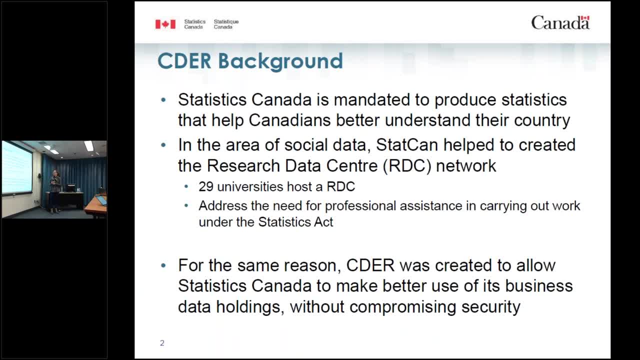 and different trends. that's obviously a very broad statement. in the area of social data, stats can help to create the research data center network- uh, i think there- i'm not sure- 29 universities, but there's 30 locations across canada- and the rdc network addresses the need for professional assistance in carrying out. 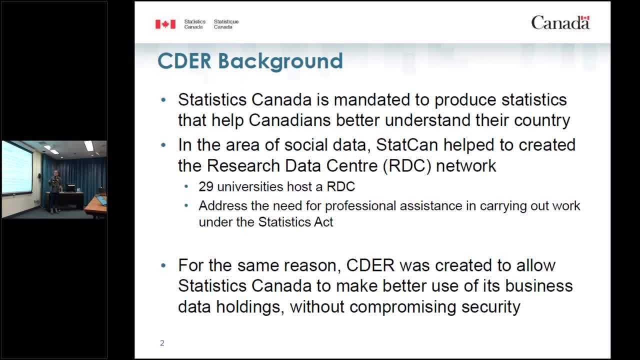 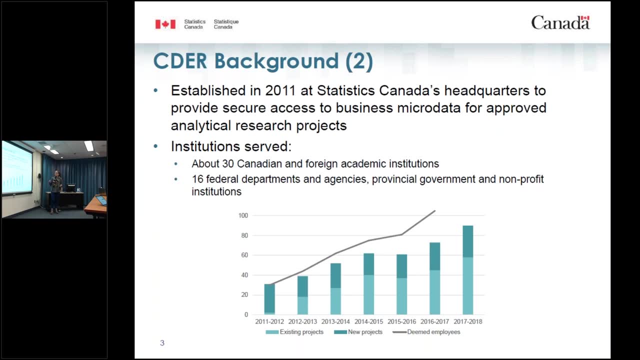 work under the stat act. for similar reasons, cedar was created to allow statistics canada to make better use of its business data holding without compromising security. so our center was established in 2011, so it's fairly recent compared to other research data centers. it is located, at the moment, only at the headquarters of statistics canada in ottawa. 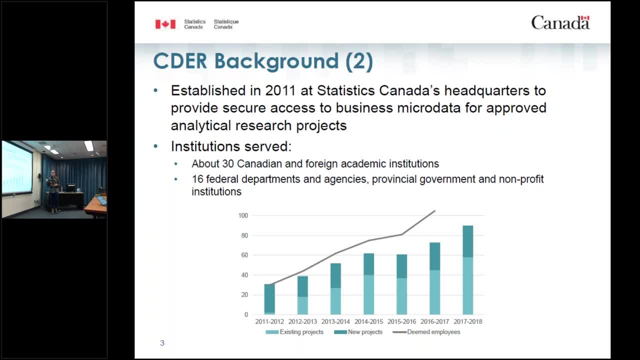 and provide a secure access to business micro data for approved analytical research project. our clients are very diverse. the researchers that come to use our data are very diverse. they come from 30 different canadian and foreign academic institutions, as well as a number of other 16 and over federal departments and agencies, provincial governments, non-profit institutions. 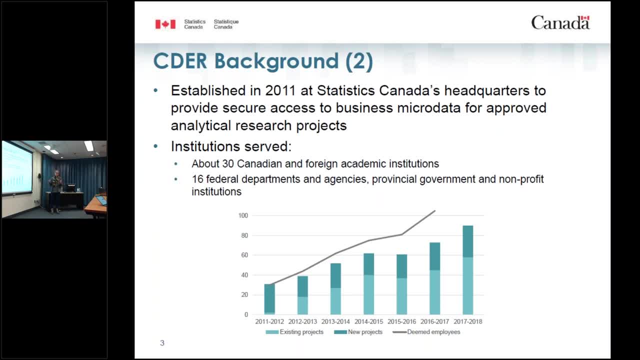 so we have researchers coming from all over the place working on different topic with the business micro data. as we can see on the graphs, it's it's opening. the research data center cedar really has seen an increase in the number of both the deemed employees or the researchers that are coming as 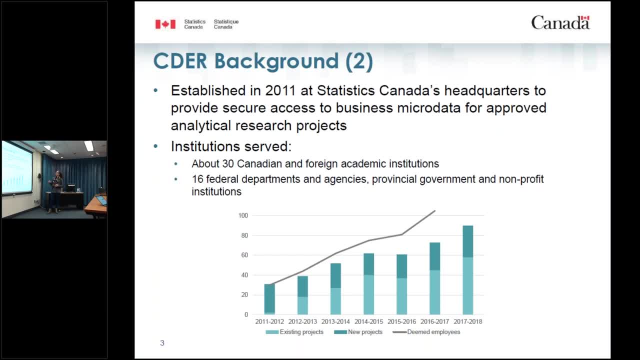 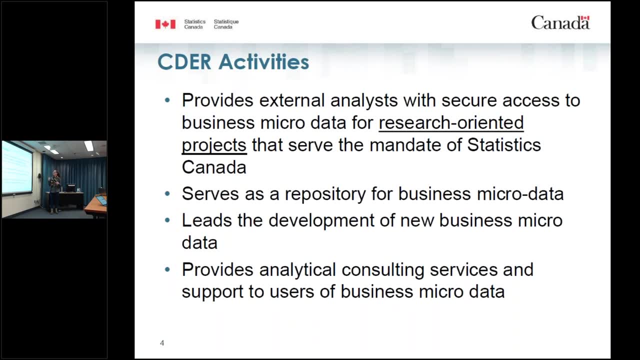 well as the number of projects that are undertaken at the center. so what do we do as a center? our activities are: first, we provide external analysts with a secure access, as i mentioned, to business micro data for research oriented projects that serve the mandate of stat scan. when 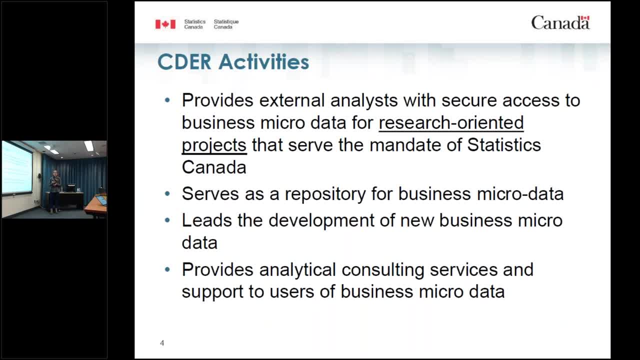 we need research oriented projects. it means that we really want to have analytical work being done at cedar. if somebody really is looking more for tabulations and summary statistics, that really isn't the the right forum for that. seeder also serves as a repository for business micro data and 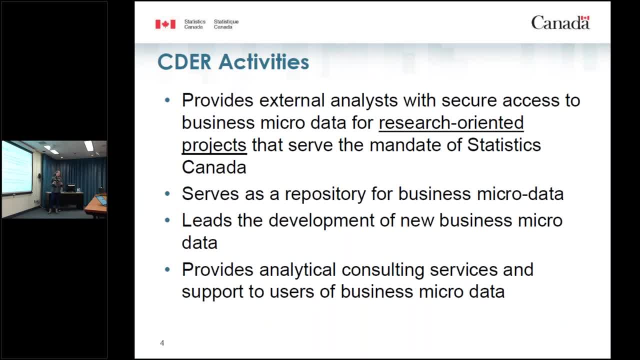 the development of new business microdata. so not only do we provide secure access to the data itself, but we also really do a lot of work in terms of developing the microdata ourselves. and finally, we also provide analytical consulting services and support to user of the business. 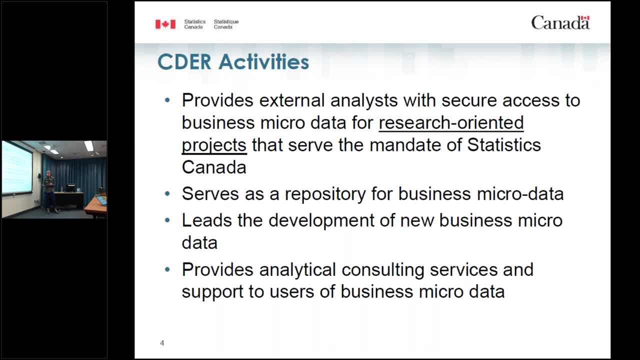 microdata. so our analysts at cedar do work with researchers and help them better understand the data, help with proposals and if they have questions about the data, they can either help them directly or be the bridge with subject matter specialist, and we also, as i mentioned, provide analytical 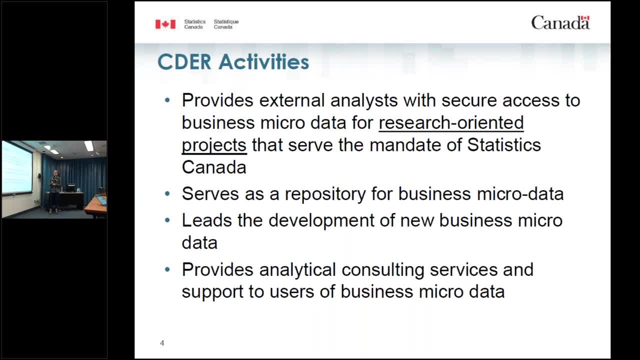 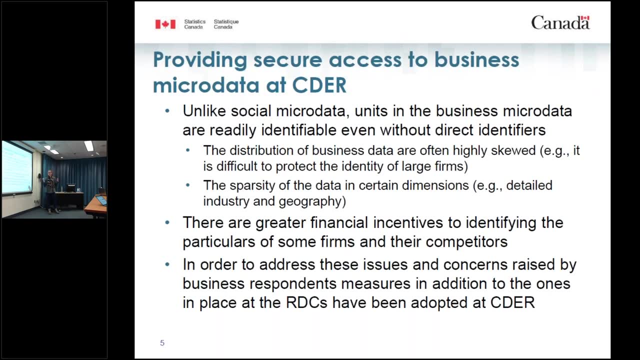 consulting services, so in some cases at a fee, at cost recovery. we also are able to do research ourselves or to prepare different statistics or reports for clients. so what do we do? why are we so special? why is the business micro data not in the research data center yet? so, unlike the micro, 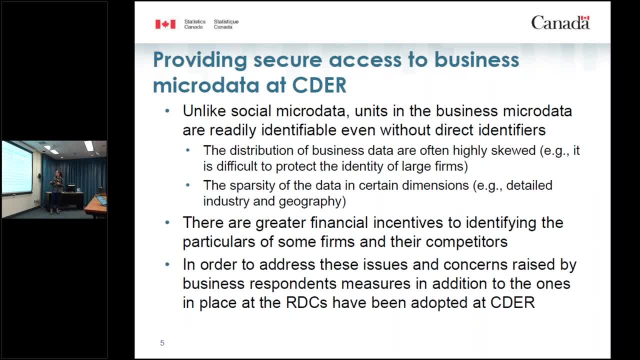 the social micro data that's in the, in the rdcs. the units in the, the business micro data, are really easy to be identified, even if you remove the name, even if you remove anything that can help identify directly the company. what happens is the distribution of the units is really skewed. 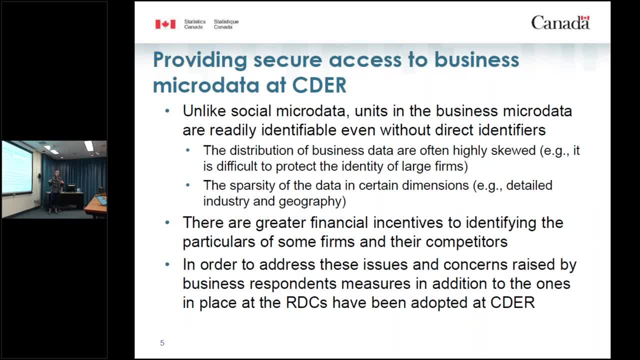 so, as we know, a lot of companies in canada can be really big and really large and they're really well known to the public as well, which makes those firms very easy to identify. also, the data is really sparse, so if you look in different dimensions- for example the ddb, which is the ddb? 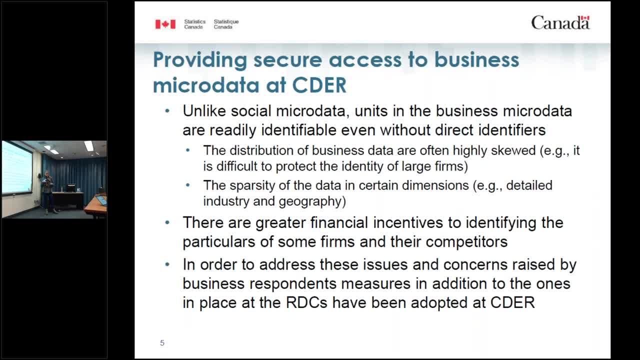 detailed geography or industry. it also provides a lot of information that can allow an individual to identify a company. For example- an example that's very easy to understand- if somebody was to look at a data set even though there's no name, no direct identifiers. 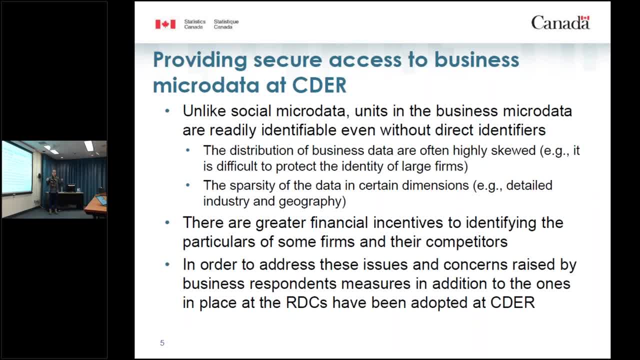 if you know that the company is located in Montreal and if you know that the company is in aerospace, there's a very good chance that you can, only, with that information, are able to identify that company and then you're able to know all of the specific information about that. 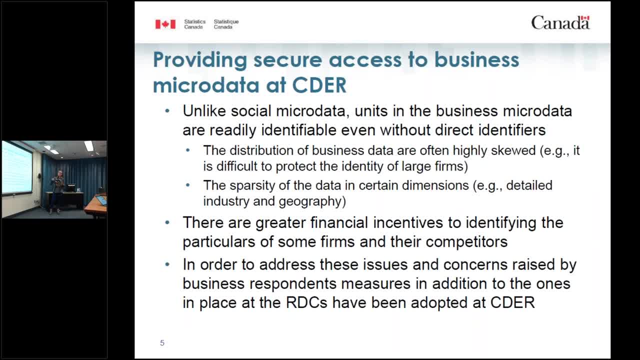 company. So that's what we want to protect. So that really is one of the factors of why this data is only at CEDAR. Another factor is that there's a greater financial incentive So somebody to try to use that information wrongfully if you wish. So you can have somebody with bad intentions who 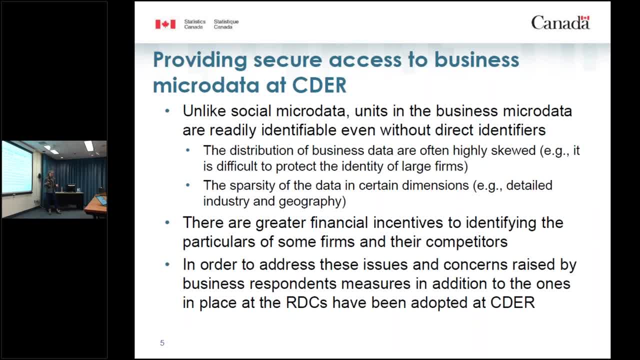 really want to come and use the data for their personal benefits, personal financial benefits. So that's one of the factors that we want to protect. So that's one of the factors benefits, or even maybe somebody has some interest in the specific companies and by 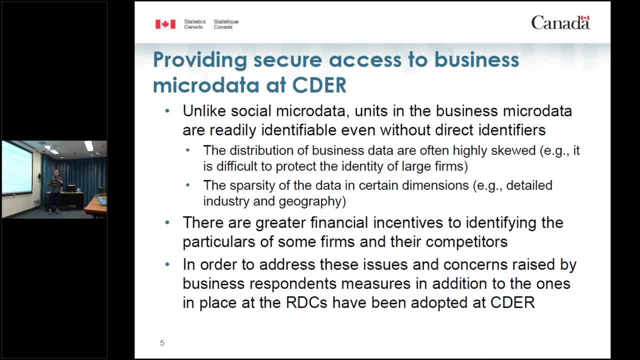 using the business micro data, they might be able to look at their competitors or look at other companies that give them some sort of information or insight on their businesses which could help them personally to have some gains. So that's also a problem which we want to really avoid. 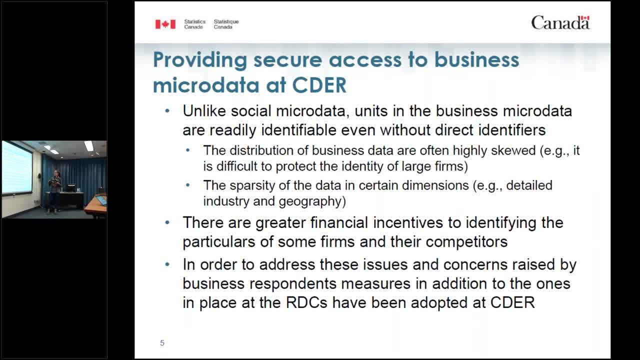 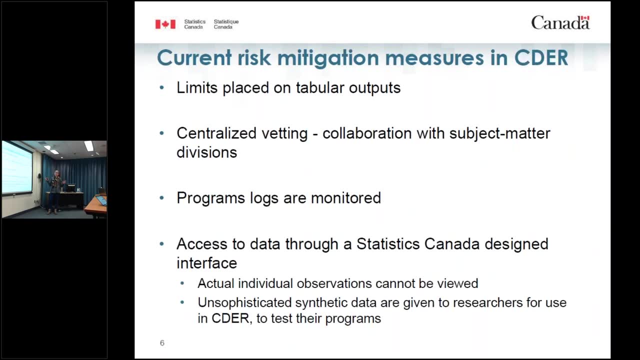 So for those reasons, the data for business, micro for businesses, is only available in our research data center in Ottawa. To address these issues, we also have additional mitigating measures that are placed at CEDAR. So those measures are: first, we have limits placed on the tabular outputs. 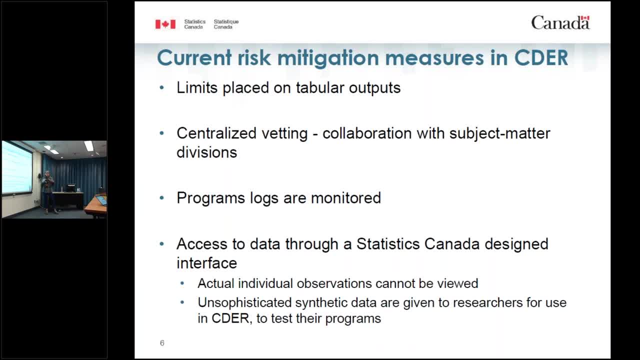 As I mentioned, it's really an access for analytical research, so people are not coming to just produce aggregate statistics. The aggregate statistics or the summary statistics that are produced at CEDAR really should be produced in support of the analytical output. We also do centralized vetting. that is done in collaboration. 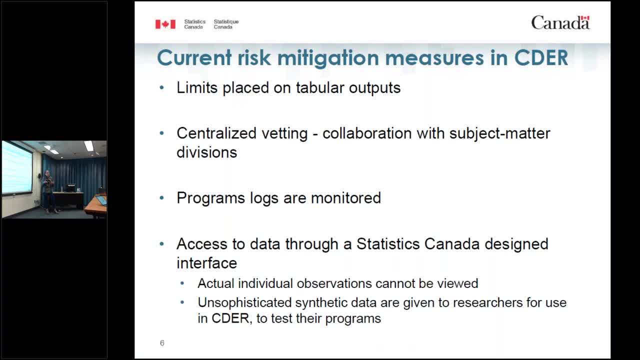 What is the vetting? It's similar to what's done in DRDC. At the end of the project the person needs to have the output or the results verified to ensure that no confidential information is present in those results. So we have our own analysts who do that, but when they work on a specific database, that 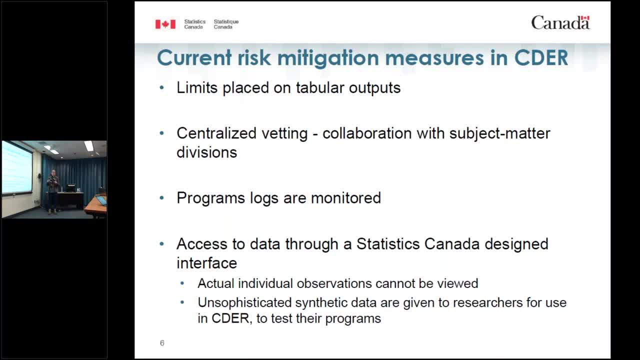 is produced by another division at StatScan. we will collaborate together to ensure that nothing sensitive is released. We also have a database that is produced by another division at StatScan. We will collaborate together to ensure that nothing sensitive is released. We also have monitoring of logs. 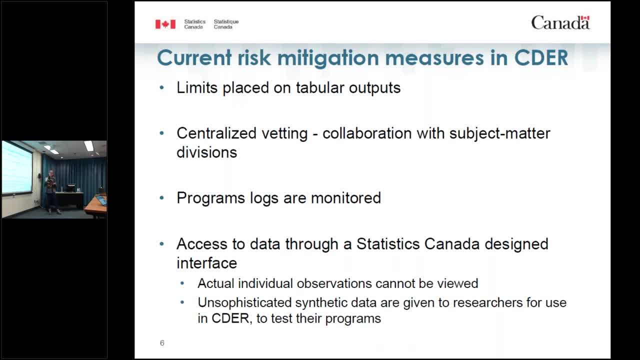 So any statalog, for example, that is produced is kept, saved and monitored for everything that is produced. And finally, and that's probably the main difference between CEDAR and DRDCs, the access to the data for business microdata at CEDAR is done through an interface. 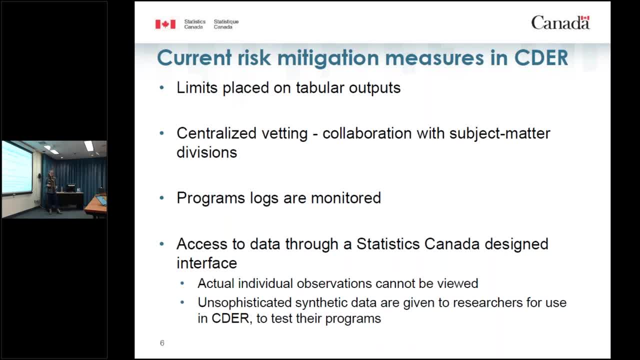 What does that mean? It basically means that even though the researchers come all the way to Ottawa to work with the business microdata, even when they're at CEDAR, they're not allowed to see the business microdata. They can only work with the data through an interface. 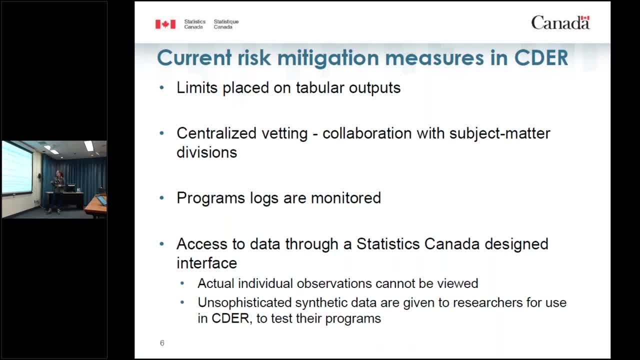 We provide them with what we call unsophisticated synthetic data, or fake data. that gives them the opportunity to see the structure of the data, understand how it's constructed, what it looks like. They can build their program accordingly. looking at the synthetic data, looking at 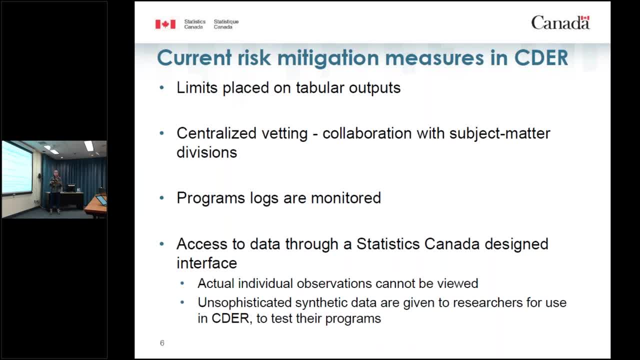 its structure. They can test their program on the synthetic data, but once they want to use them on the real data, they have to send the program through. They have to send it through an interface and then they receive the results automatically in real time, without ever seeing any individual observation. 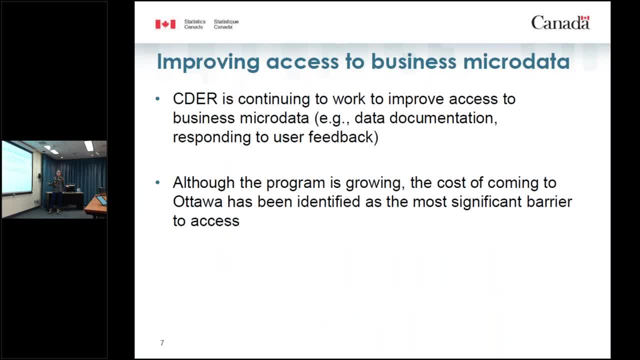 At CEDAR. obviously, we want to open the access to business microdata and we really want to improve the way that we are working. Some of these things are small. well, they take time, but you could see it as a smaller. 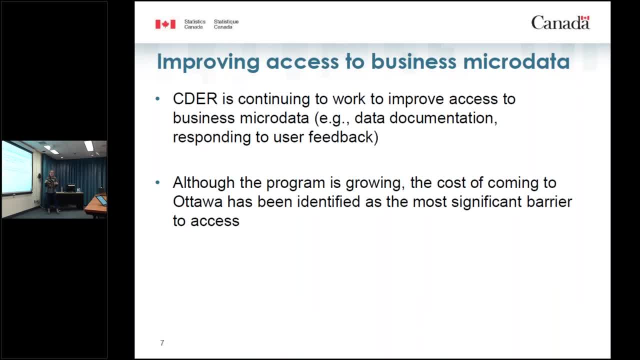 initiative, For example, improving our data documentation to ensure that people can access the data. people have to know what is available and what is out there. So we've been working a lot in the last year to improve our data documentation. We're talking about record layout, data dictionaries, user guide on our different data sets and 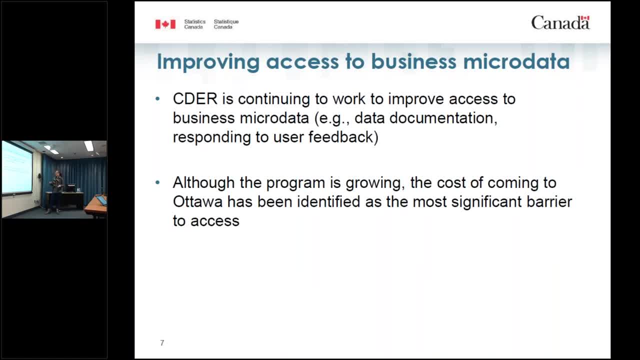 the hope of putting it on our website so that people really know what's out there and what is available, so that it helps them build their proposals. Also, we try to respond to the user feedback that we get. So we really like to interact with our user and really like to get feedback, good or bad. 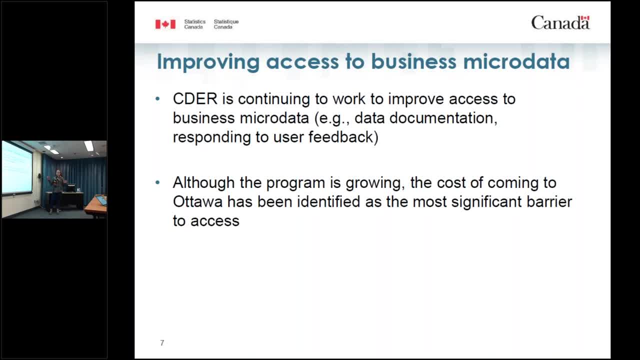 so that we know where we have to go, what needs to be improved, Amongst other things. we have a lot of people that are really interested in this, So along those feedback, we've realized since the start of CEDAR that one of the biggest 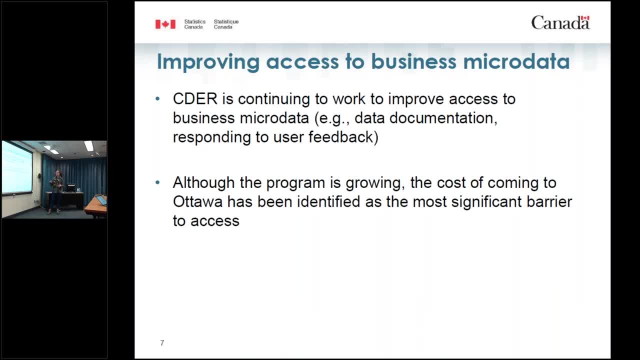 barriers to access of business microdata really is coming all the way to Ottawa. Obviously, there is a big cost. If there's a student from UBC and they want to come and use our micro business data for research, it means that not only do they have to pay for their access at CEDAR, but they 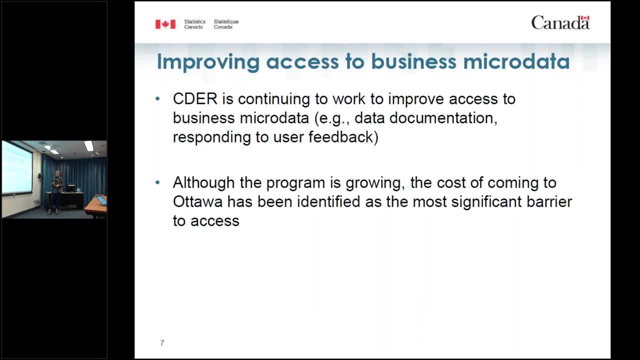 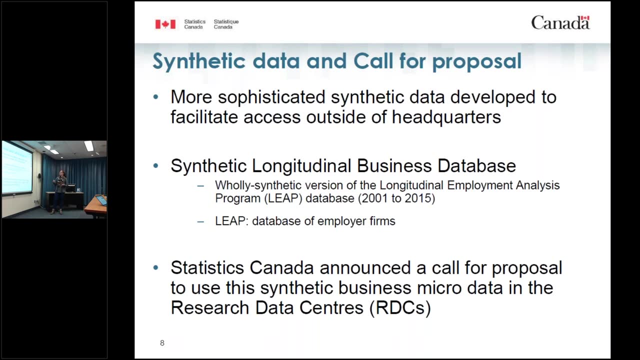 also have to pay for a flight, for a place to live at the same time, and it really can create something that is not possible for some research. So what have we done to try to alleviate some of these concerns? We've been working on synthetic data and recently, in March, early March- we have put 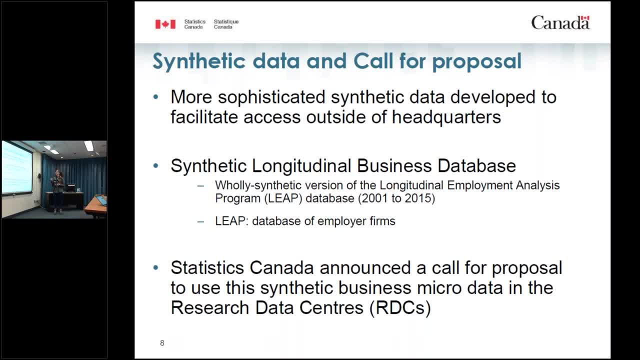 out a call for a proposal. So what we've done is more sophisticated synthetic data developed to facilitate the access outside of headquarters. It's a synthetic functional business database, which means it's a wholly synthetic version of LEAP, the Launchable Employment Analysis Program. 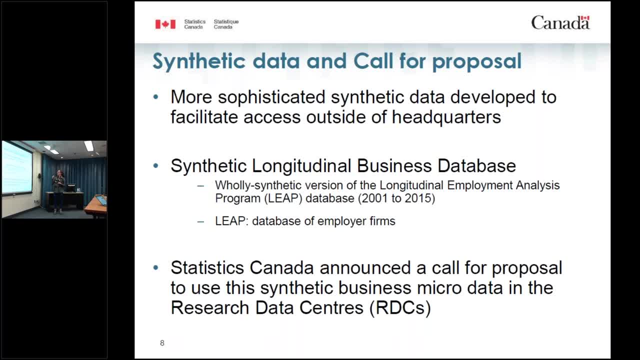 From 2001 to 2015.. What is the LEAP? It's basically a database that includes all of the employer firms in Canada. So one might ask: well, you already have synthetic data in CEDAR. What is the difference with this and why are you putting synthetic data or creating? 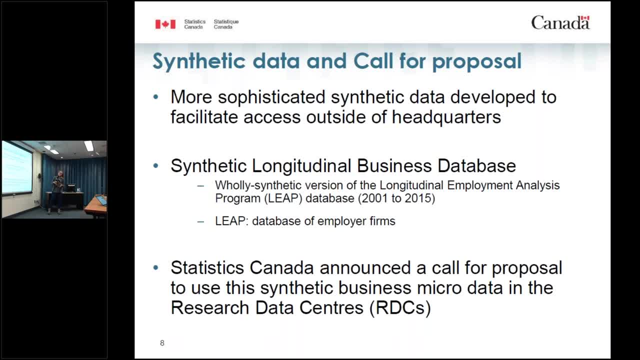 or spending so much time on this one to put in the RDC. At CEDAR, the researchers who come have a really close relationship or a big proximity with our own analysts, our analysts that are able to see the real data, that are able to 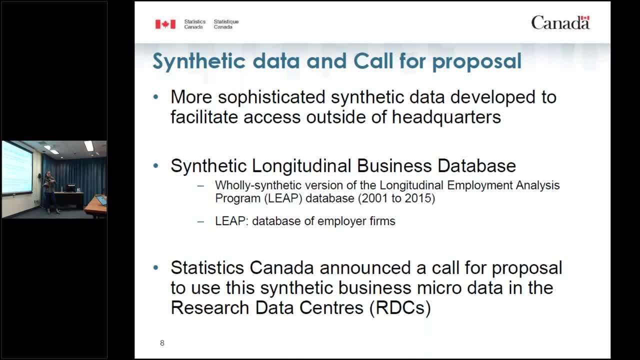 help and answer questions in real time, And so I would say that the quality or the closeness, if you wish, of the real data versus the synthetic data doesn't have to be perfect, because you have people on site to really help and answer questions. 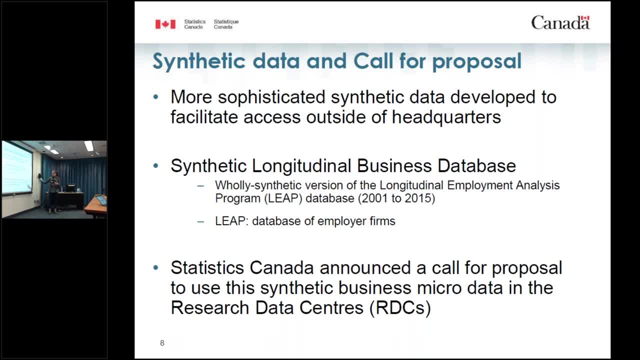 What we want to do by opening the microdata and putting it in the RDC. when we do this, it means that the researchers will go at a remote location in an RDC and use the synthetic data To be able to use it without having really the more difficult interaction with people. 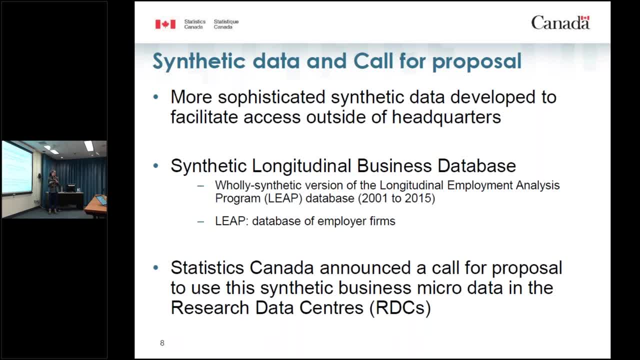 with people that are based in Ottawa. we want to have something that is really much closer to the synthetic data, so that researchers really are able to build their programs and make some decisions on their analysis based on the synthetic data. And so, after we've been working on all of this development for synthetic data, StatCan 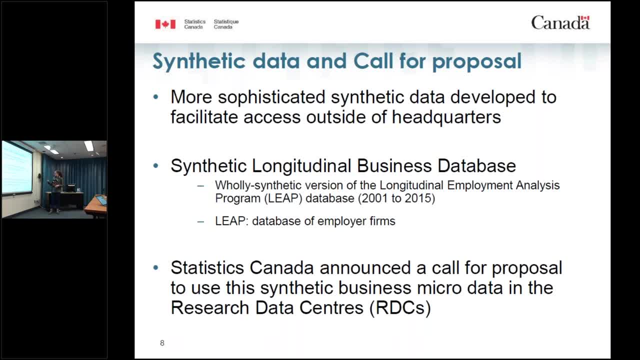 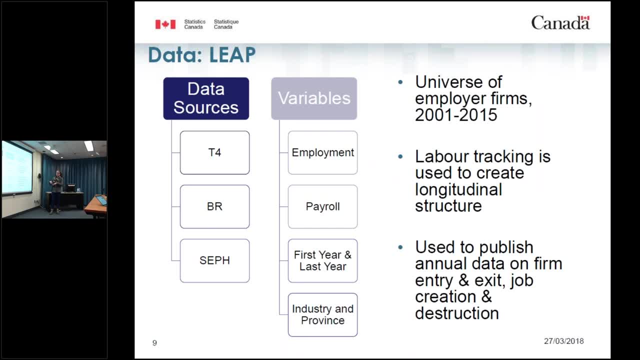 has announced a call for proposal to use it in the RDCs. So what is LEAP? LEAP is a database that's been around for many, many years. It was created in the 90s, so it's a really old data set, which means it's good quality. 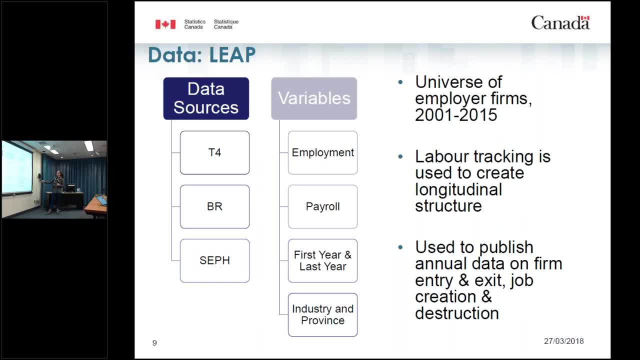 and it's been used by many researchers on many different topics. How is it built? There are different data sources. The T4 of remuneration paid, which is basically what we all fill, or all receive, I should say, for our tax purposes. 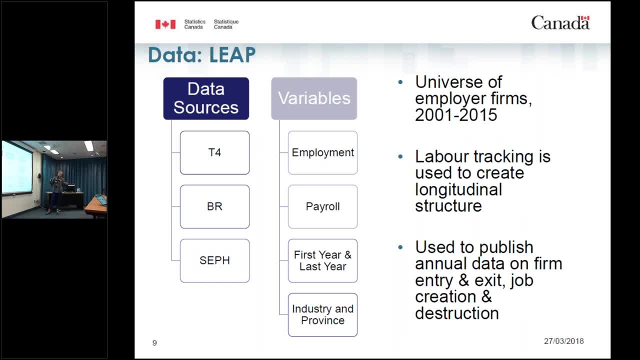 The business register. so the BR, the business register, is a database or, if you wish, yeah it's a database, but it really is a database that shows the structure of all companies and all enterprises in Canada each year. It's very complete and includes a lot of information on companies, for example, their ownership. 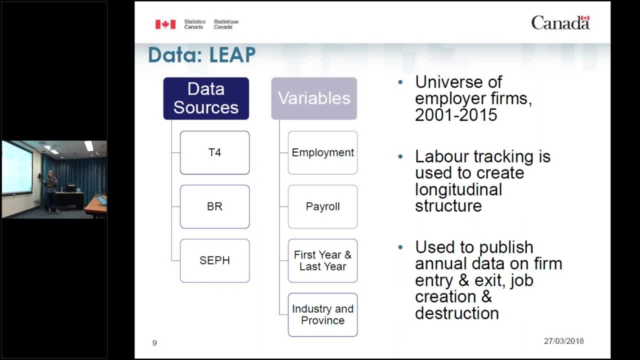 if it's foreign or Canadian, the industry of the company. so there's a lot in there. And last, we also use the survey on employment and payroll and hours in the construction of LEAP, which help us to really design and derive a measure of employment based on T4. 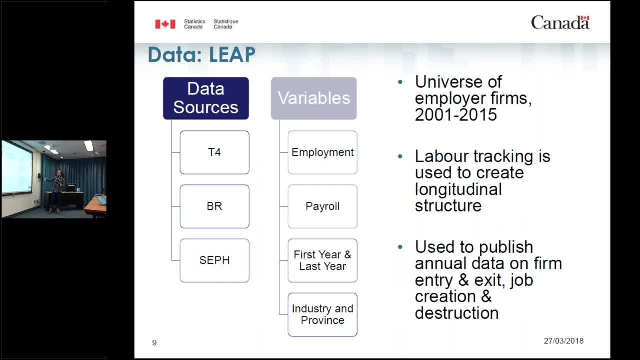 and SES variables With all of these. So what we get in LEAP we have variables including employment, the payroll, the first and last year of all companies, so we're able to find when they enter, the entries as well as the exits, and we also have information on the industry and the province of the company. 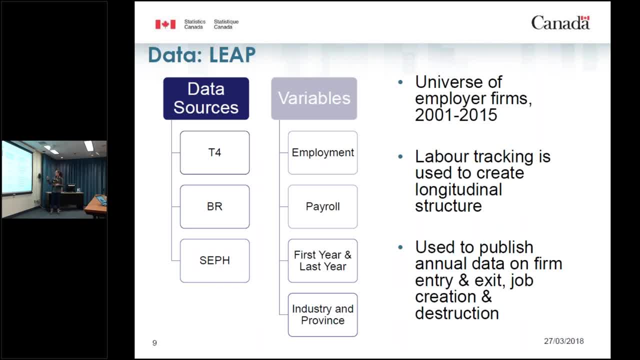 So it's really, as I mentioned, all of the employer firms in Canada. One other feature that is fairly interesting from that database is that it is longitudinal. It is longitudinal because we are using labour tracking to make some connections for firms that might have a broken history. 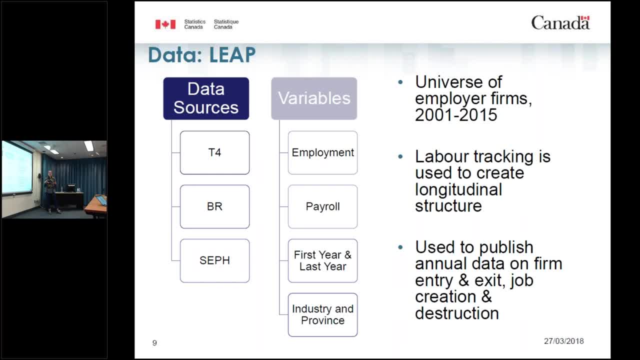 What do I mean by that? Sometimes firms will have some administrative change. maybe they decide to change their name one year and maybe this creates a break in history, because you have the firm with its first name for a few years and then it changed name and we have a new history. 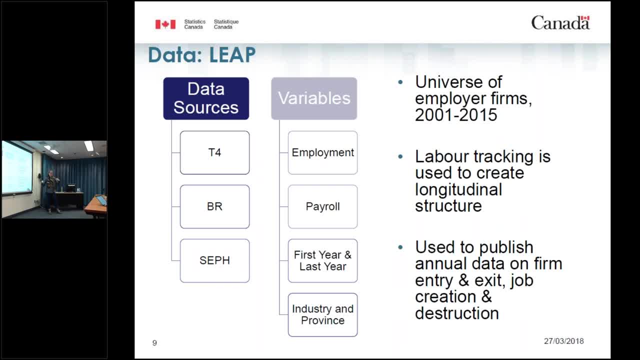 So in the data set- an administrative data set- it could look like one firm died and then a new firm was born. What we do is by looking at all the employees that are in that company. if we find 90, 100%. 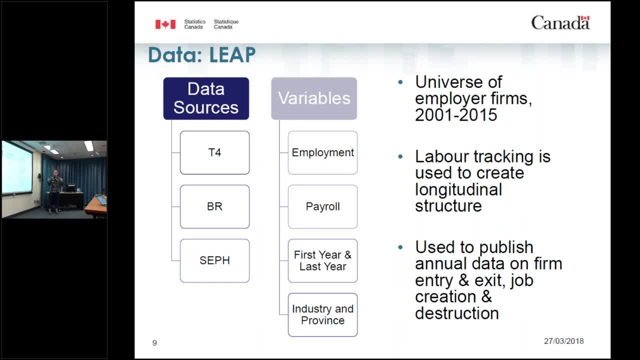 of these employees in a new firm the next year, Depending on the size of the company. we're able to make decisions to make sure that we re-recreate, not recreate, but that we connect these together to ensure that we have a longitudinal set. 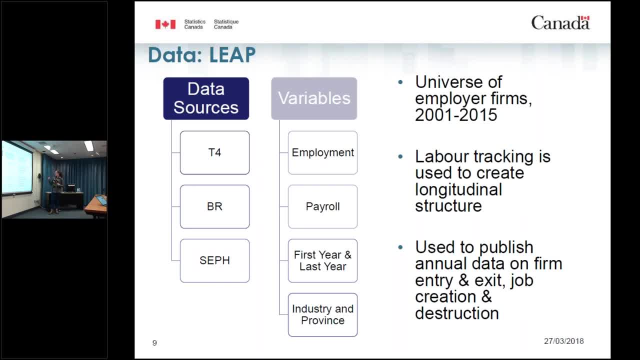 And how is it used? Where is it used? That's that scan the leap Right now. what we're doing with it obviously research and access, but we also publish CANSIM tables on entry and exit of firms, as well as job creation and destruction. 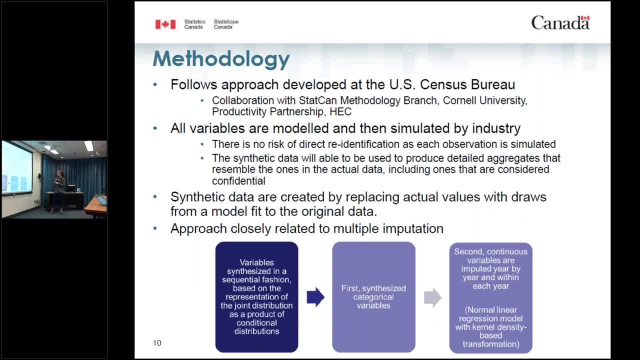 So, precisely, or more specifically, what is it? What is it? What have we done with the synthetic data and how have we created it? So the methodology that was used was not an innovation of StatScan. The work that was done to create that new sophisticated synthetic data was really collaboration. 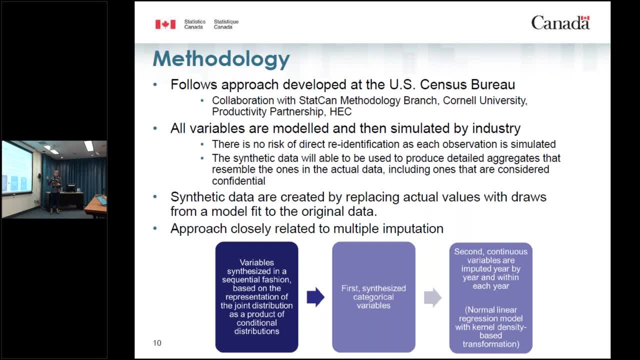 So we followed an approach that was developed at the US Census Bureau and they have a synthetic longitudinal business database now that is used in the US following that methodology. So for this project we collaborated with the StatScan methodology branch Cornell University, the Productivity Partnership, as well as HSE Montréal. 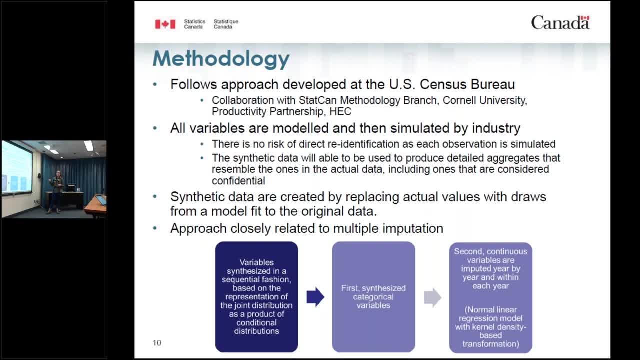 All the variables are modeled and then simulated by industry, so there is no risk of direct re-identification because all of the observations are simulated. The synthetic data is also able to reproduce very closely aggregates from the actual data, which means that a researcher can do it. 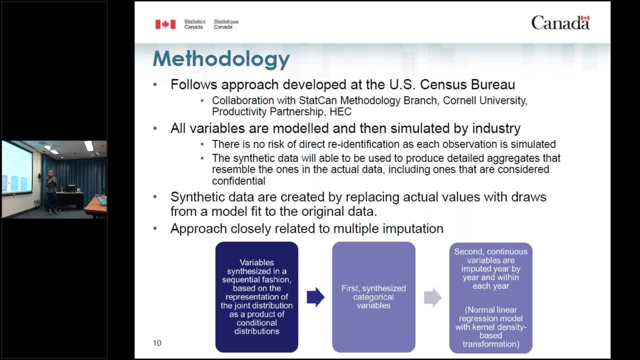 So researchers working with the synthetic data, trying to make summary statistics, different totals, will have information that will be very close to what one would get from the real data. The synthetic data is created by replacing actual values with draws from a model fit to the original data, and it's an approach that's closely related to multiple imputation. 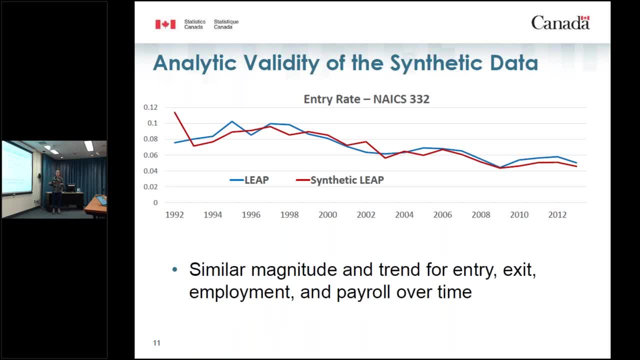 Once the data was created, we've done some tests to determine if the synthetic data was analytically valid. So one of these is, for example, looking at the different trends that we see both in the synthetic and in the real data. So on this graph, on this chart, you can see, for one specific industry, the entry rate of 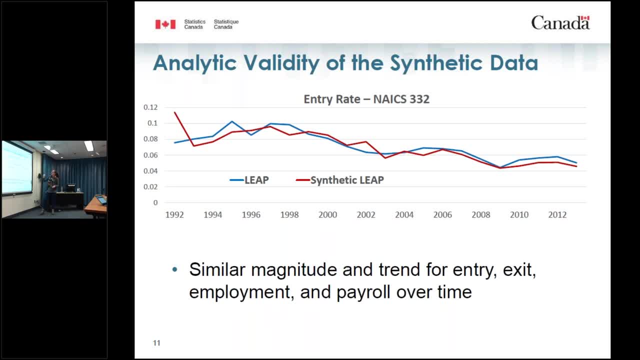 companies in each year, so the number of new firms each year We see on the blue line that's based on the real data and the red line is based on the synthetic data. So they are different, as they should be, because one is fake and one is real data, but the 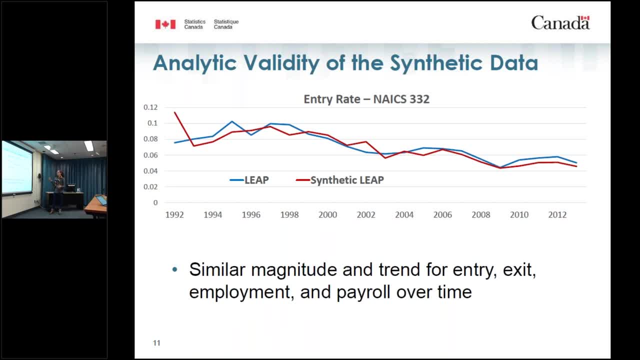 But the trends that are shown, and the magnitude as well, are very similar, which shows that we kept. really, while the data is synthetic or fake, it's very close from the original data. This type of test was also done not only for entry, but as well for exit trends in employment, payroll as well, over time. 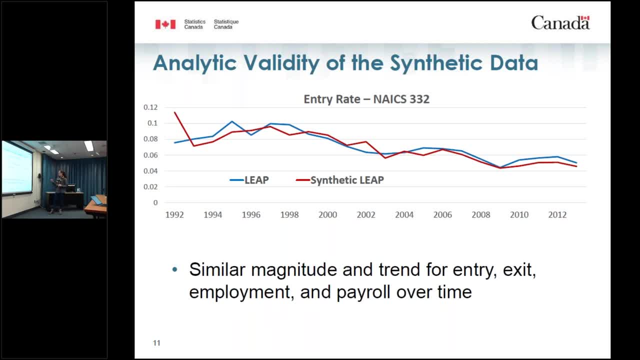 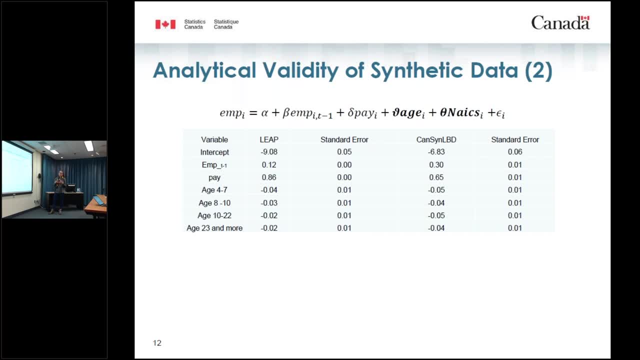 And we also get similar trends. Another way to look to see if the data is valid and if relationships are kept within the synthetic data compared to the real data is doing some regression analysis. So this one is obviously a very simple regression where we have employment, one year, employment in T-1, the pay age of companies and the detailed industry. 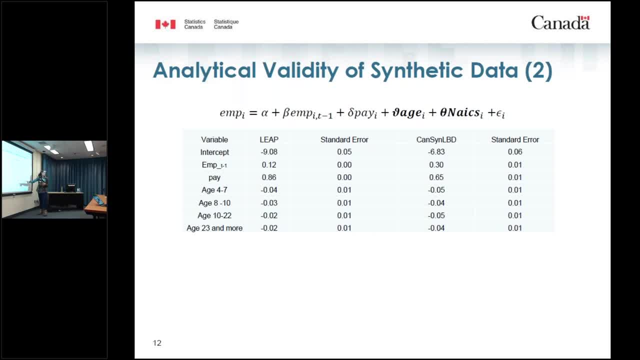 So we have the coefficients here. We didn't put the industry coefficients for confidentiality. Oh, I see. So, yeah, thank you. So we have all of our variables. So here we have the coefficients for the real, And here on the right side we have the coefficient for the synthetic data. 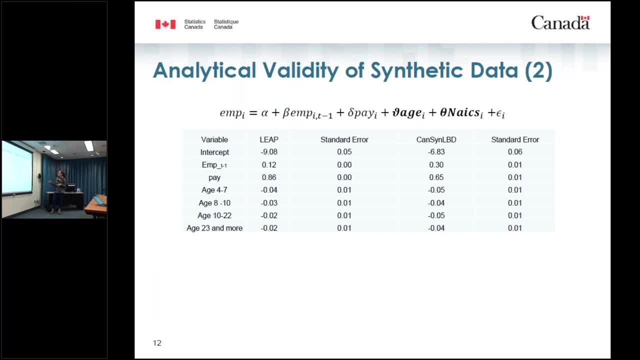 While the coefficients on one side and compared to the other side, the magnitude is different. the direction of the coefficients, however, is the same, which show that relationships are maintained, which is what we're looking for: to ensure That it's robust and that somebody can at least design their analysis based on the synthetic data. 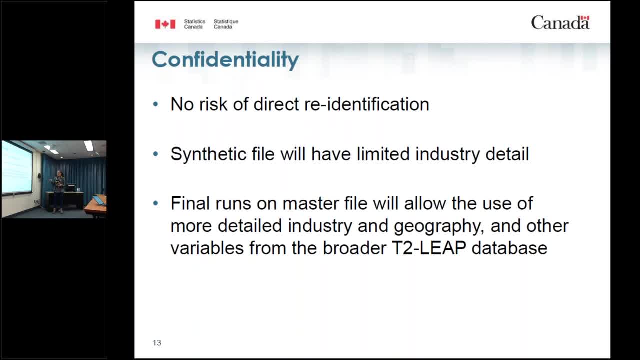 So with the synthetic data there is no risk of direct re-identification. The synthetic file that it produced would have limited industry detail And final runs are done can be done on the master file and can allow a more detailed use of or the use of more detail of more detailed industry and geography, as well as other variables. 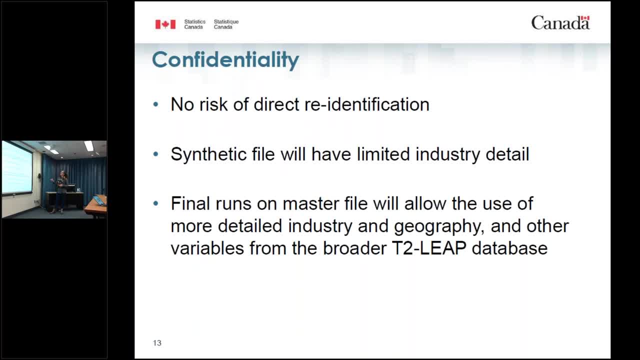 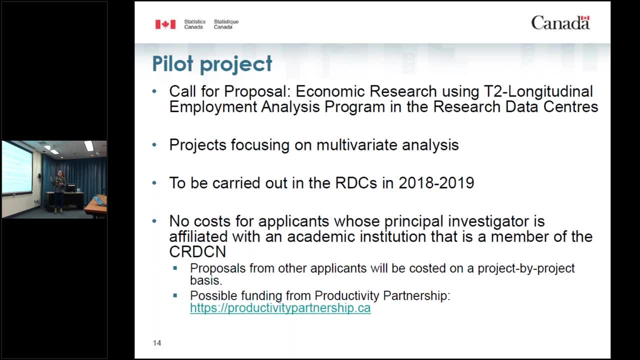 And we look at these variables from the broader T2 leap So to include T2 variables. So this pilot project- So I mentioned I had this call for proposal- the pilot project really is using for researchers that want to do economic research using the T2 leap in the RDC. 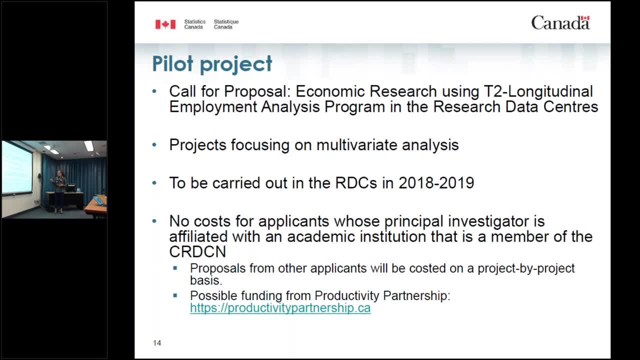 We are looking for projects that are focusing on multivariate analysis, and these projects should be carried out in the RDC in 2018 and 19.. For applicants whose principal, whose principal is Democratic and studies research- And this is a focus here, I think, for the RDC. 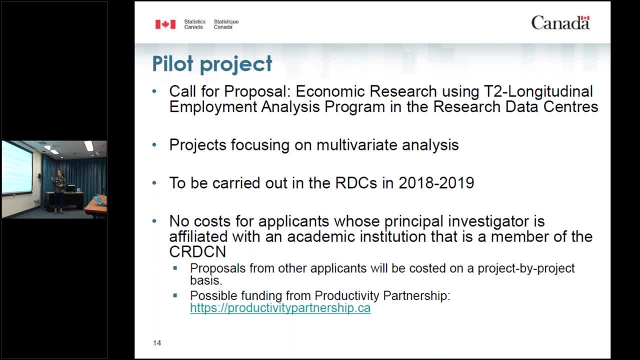 And this is looking at researchers who want to do economic research For applicants, whose principal, For applicants who's principal investigator is affiliated with an academic institution that is a member of the CRDCN. there would be no cost, which is a big plus, I believe, for this pilot. 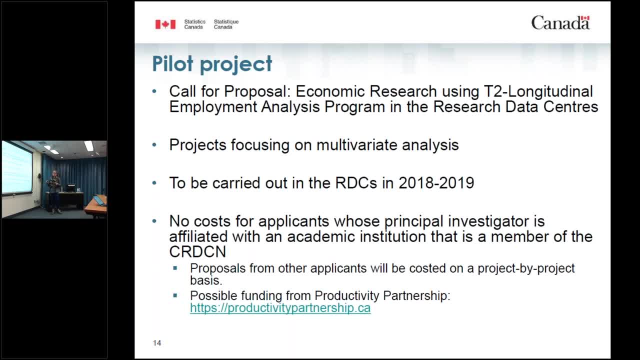 For proposals from other applicants. the cost will be determined on a project basis, project by project basis. Also, I should mention there is possible funding available from the Productivity Partnership. The website is down there, so the Productivity Partnership can offer funding not only for accessing the data, but 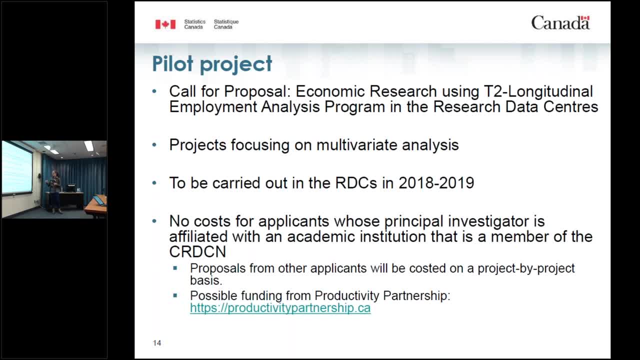 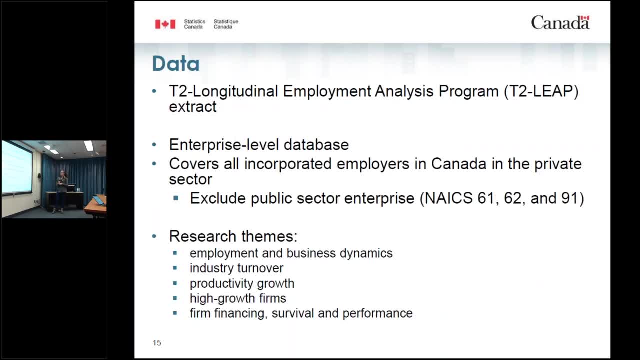 as well for different if you need for travel, for example. There's a lot of information on the website and I invite you to go and take a look at it. So our data, The T2Leap, as I mentioned what it is. So it's an enterprise level. 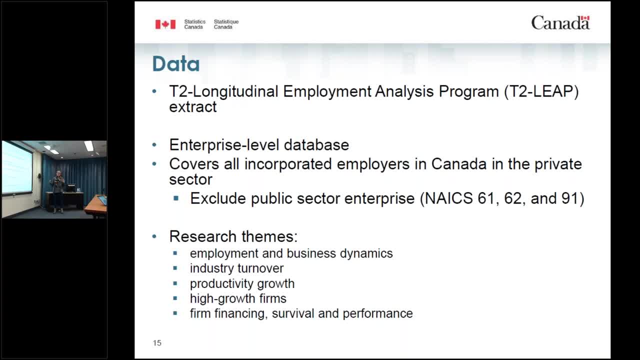 database, so it's really at the enterprise level. This means that if an enterprise has multiple establishments, we will only have information for the whole enterprise itself. The database has a very big universe. It covers all of the incorporated employers in Canada in the private sectors. so we exclude the public sector by excluding companies. 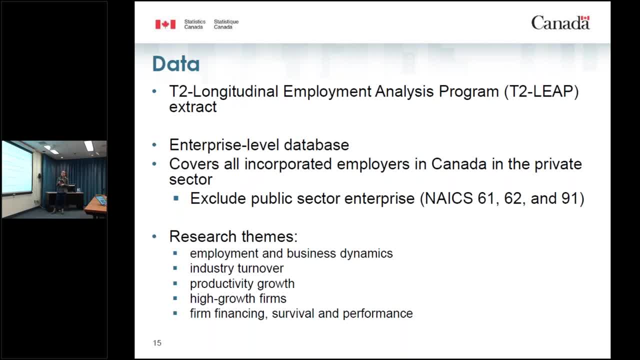 that are in the age of 61,, 62 and 91, which are health, education and public administration. In the past, well, T2Leap has been around for a very long time and so in the past, the research that has been done has been looking at. 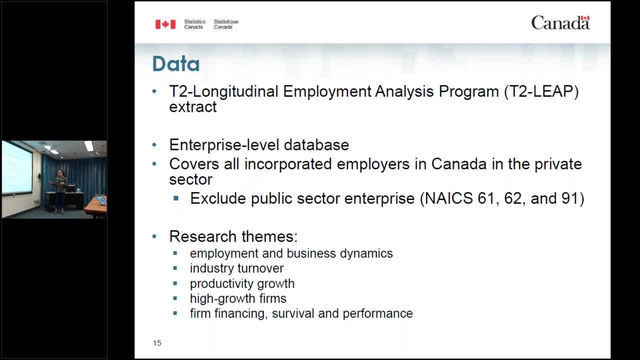 employment and business dynamics, industrial turnover, productivity growth, high growth firms from financing, survival and the like. O'Reilly Network, our business network for Sustainability Development, is a diverse, high-rise enterprise with highly-tốn trading funds. The details andickt are shared in the video manufacturer and livelihoods are provided for all. 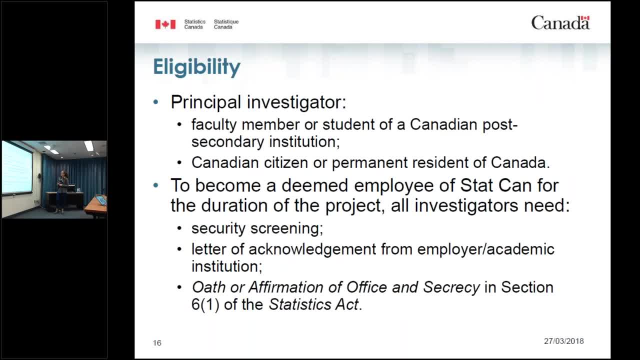 and performance, So all of these are possible to look into. For this specific pilot, the eligibility of researcher is what we're looking for. The principal investigator should be a faculty member or a student of a Canadian post secondary institution As well. the principal investigator must be a 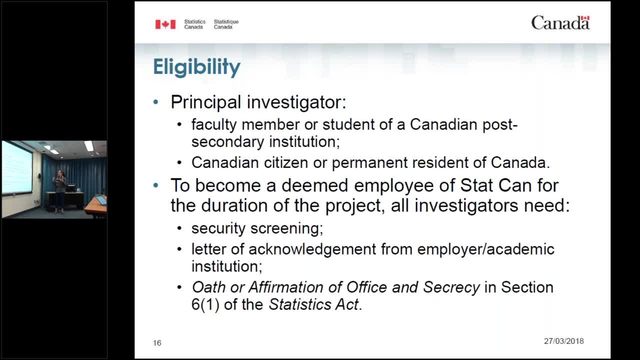 Canadian citizen or a permanent resident of Canada To become a deemed employee of STATSCAN for the duration of this project, all investigators need to go through a security screening which is similar to what is done in the RDCs. They also need a letter of acknowledgement from their employer or 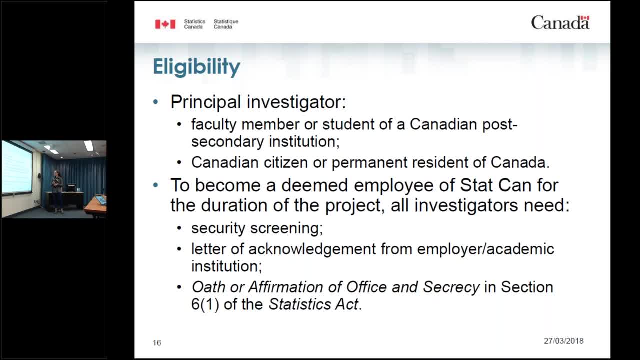 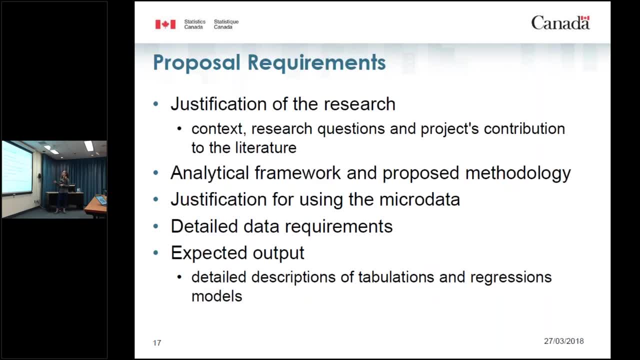 their academic institution and they need to take the oath of affirmation and secrecy related to the Stats Act. What we're looking for in the proposals for this pilot: First, we need a justification of the research, the context, the research question and how the project contributes to the literature. 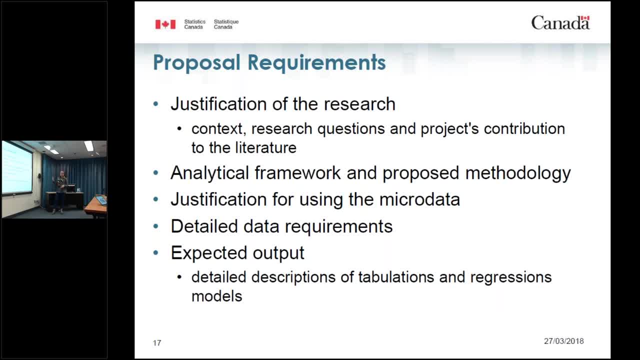 The next. we also need details on the analytical framework and the proposed methodology. One that's important is also the justification for using the microdata. So why do you need to access the microdata? We want to make sure that if you are applying to use this microdata, it means that it's 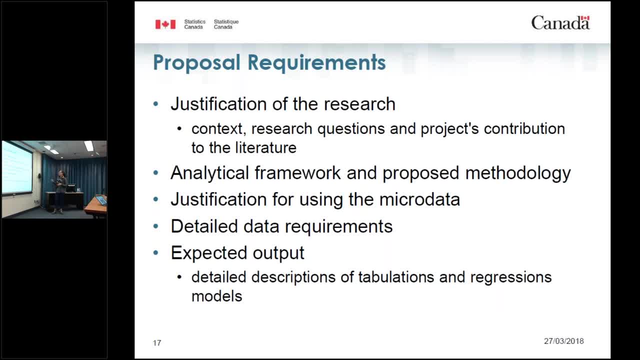 impossible for you to do the similar research with aggregate data. We want detailed data requirement And, finally, expected output. What we mean by expected output is a detailed description of the tabulation and the regressions that are going to be taken out at the end of the project. We also need details on the 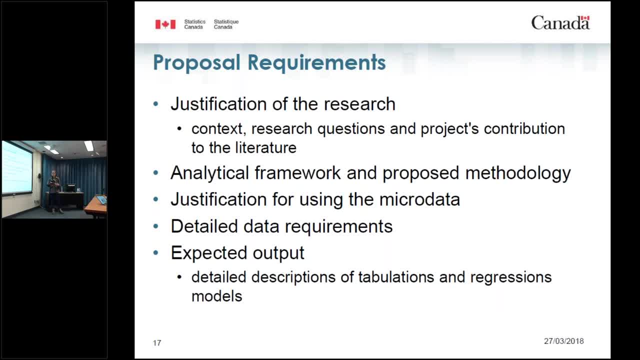 project. We do understand that those can change somewhat as the research advance and progress and once you use the data, But we want to have an overview of the quantity of output that is expected, as well as what is expected in general, How these proposals are. 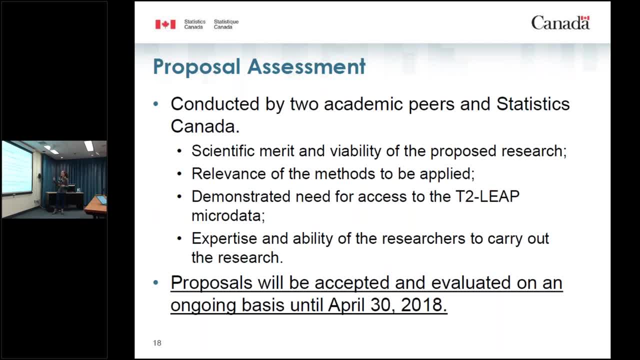 going to be assessed and how are we going to decide who's going to participate into the pilot? Well, I should mention that the assessment of all the proposals will be done not only by Stats Gantt, but as well by two academic peers. The criteria that are going: 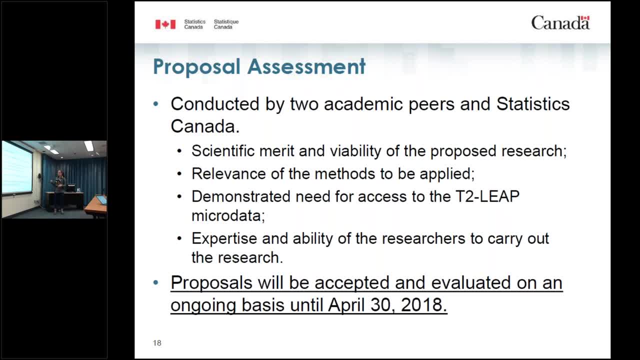 be evaluated are scientific merit and viability of the proposed research. so we want to make sure that the research is feasible, the relevance of the methods to be applied, we want to demonstrate a need for access to the T2LEAP microdata, as I mentioned previously, and we want also 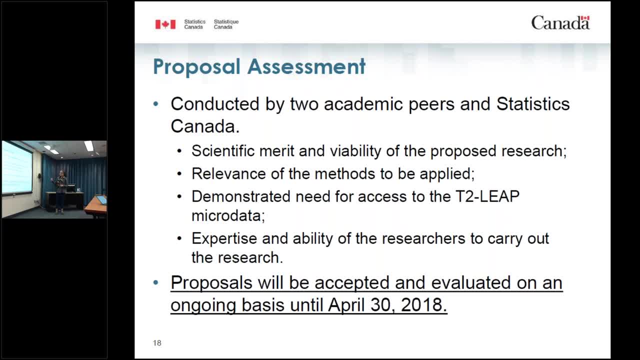 to ensure that the researchers have the expertise and ability to carry out this project. So the proposals for the pilot will be accepted by CEDAR and evaluated on an ongoing basis until April 30, 2018, so there's another full month before the end of the call for. 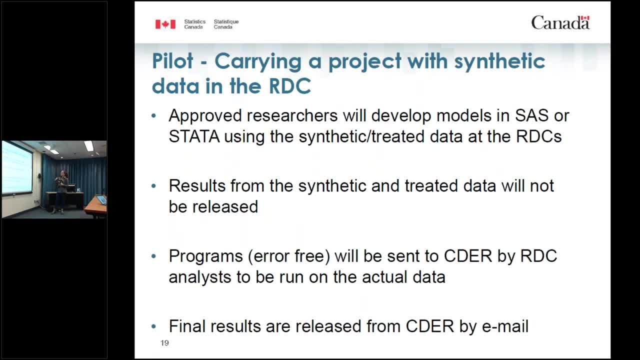 proposal. So the pilot, how is it going to work? So we've talked about it. we've talked about the proposal, but how is it going to work with the synthetic data versus the real data? So the approved researchers will be able to go in the RTCs and use the synthetic data. 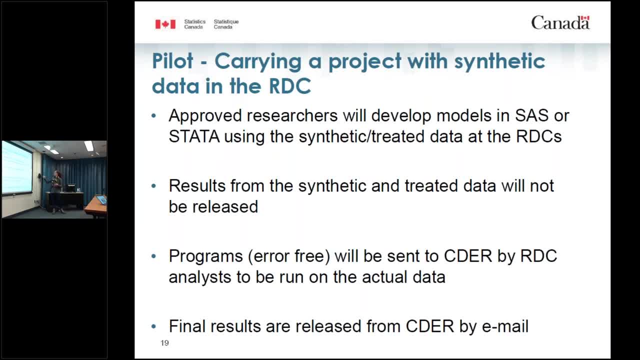 to develop their programs and their analysis. They will be using SAS source data. Those are the two language programs that we are offering for this pilot. While they test their programs and everything and doing the research on the synthetic data and the RTC, researchers will get results on the synthetic and treated data, but those 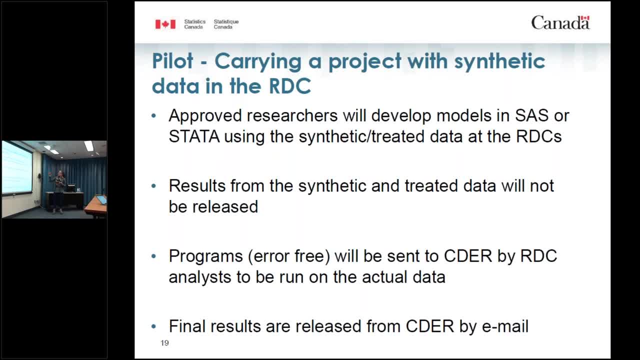 results will never be released. Those results really are used to build the analysis. Once the researcher is happy with his analysis and his programs and they go well through the synthetic data, they're error-free. these programs will be sent to CEDAR by the RTC analyst and then CEDAR's analyst will run the programs on the actual 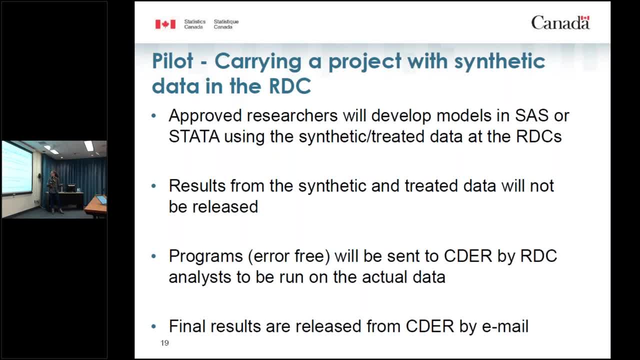 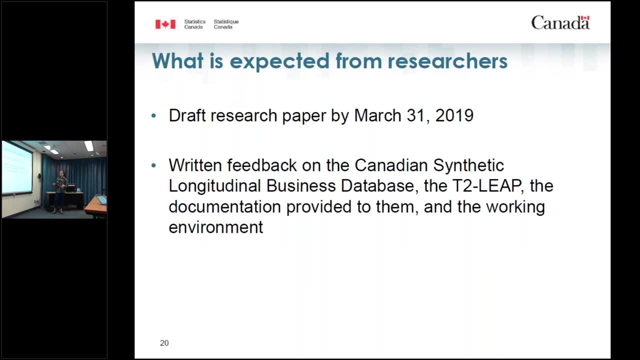 data. The CEDAR analyst will then make sure that the results are in a confidential and will release the results to the RTC analyst, which will then give them to the researcher itself. It's a pilot, so this is really obviously to test the method, test the synthetic data. 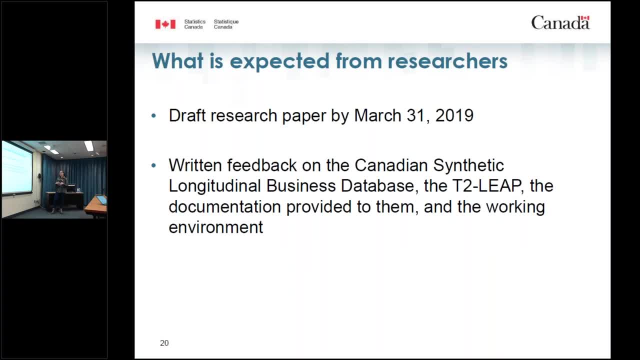 and see how it works. So we're going to test the method, test the synthetic data and see how it works. So we're going to test the method, test the synthetic data and see how it works So that we can open it in the future and hopefully introduce new and other business. 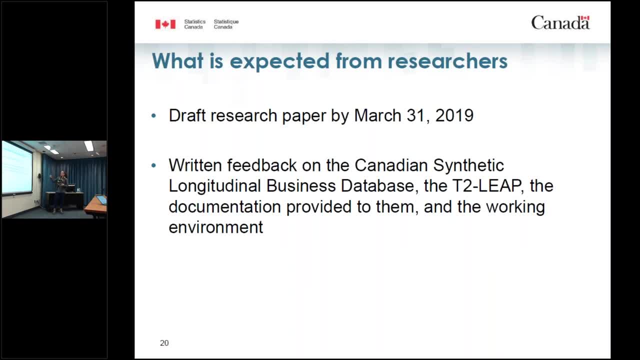 microdata as well in the RTCs. So what we expect from researchers is first a draft of a research paper by March 31, 2019.. So it doesn't have to be a complete paper or a final paper, but at least a draft to. 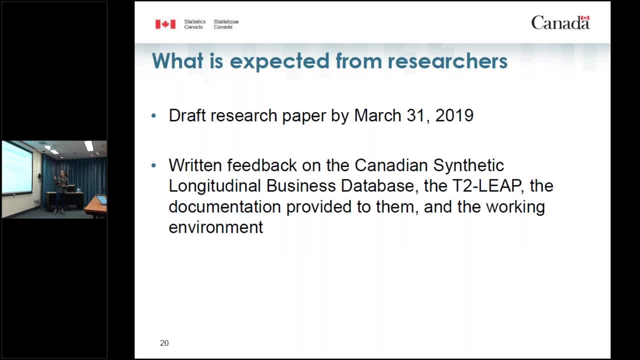 really show what has been done and how the data has been used. Also, we really are looking for written feedback on the Canadian Synthetic Launchable Business Database and the documentation provided. So at the end of the project- and I should say all through the project, we really are 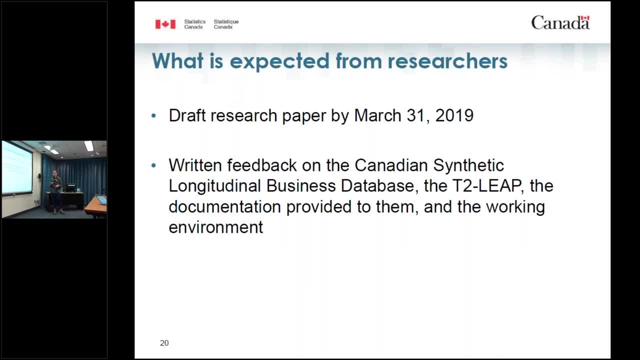 looking for written feedback on the Canadian Synthetic Launchable Business Database and the documentation provided. So we really are looking for feedback from the users. We want to know if the documentation was appropriate, if anything was missing. how was it with the collaboration and the environment? was it taking too much time? was it going well? what? 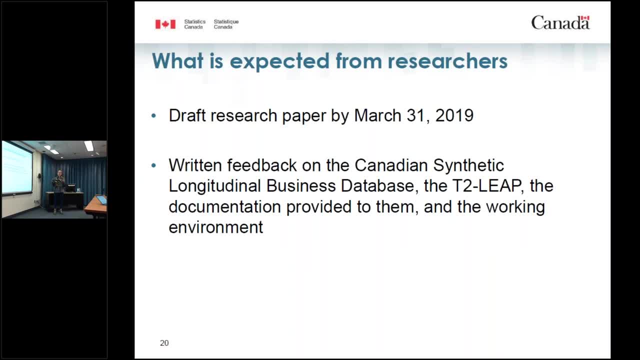 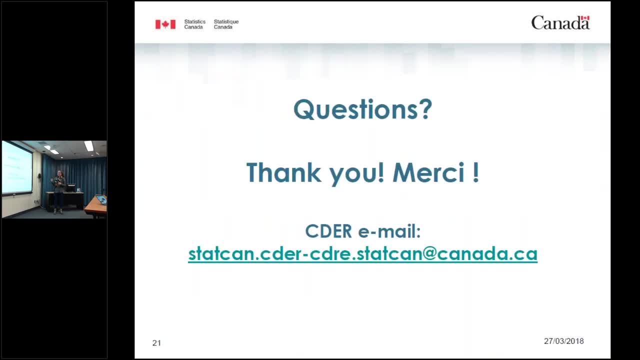 can be improved. So we want to have really an overview of the experience of the researchers working under that pilot, And that's it. So I hope that this answers your questions and I'm happy to take any more questions that you may have, either on the pilot, the data or in the RTCs. 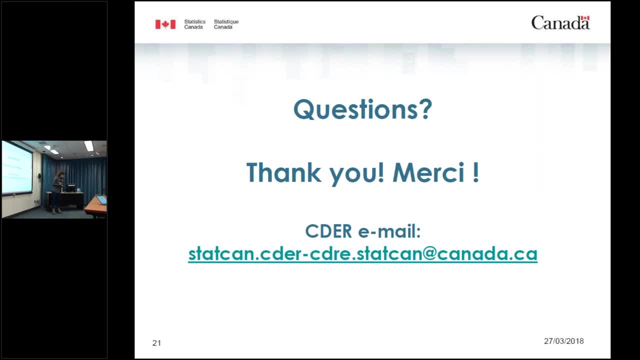 any other data set that we may have at CEDAR. Thank you, Giselle. You're welcome. That was efficient. I just sent a message to the chat to all the participants saying please write your question here. What I meant to say is write your question now. 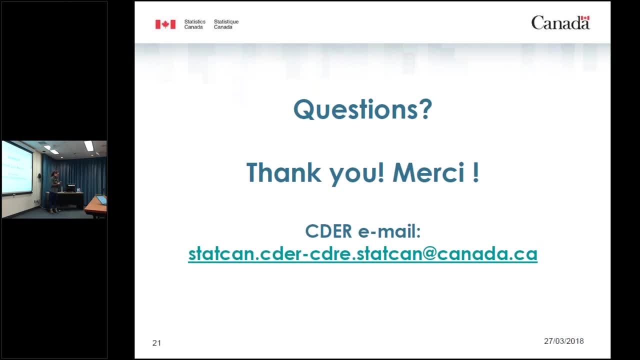 But you can either actually use the chat to ask your question, but you can also, and maybe preferably, use the question tab, and you have a space there to ask your questions. So I'm waiting for you guys And I have actually- yes, actually just. 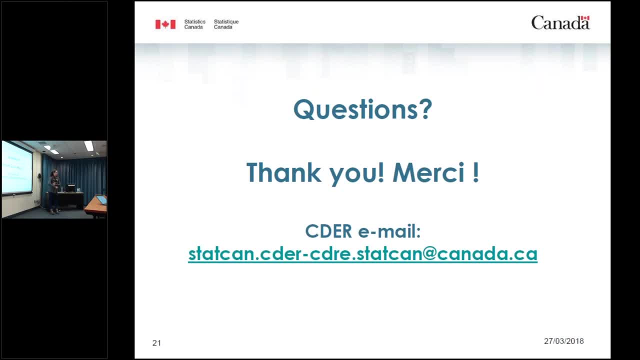 wanted to mention that, Angela. sorry, Angela, I'm going to open this thing to see everything. Yes, Angela DiNello sent me a message to explain that the Productive Partnership you mentioned that there would be fun available, And she's mentioning that actually they. 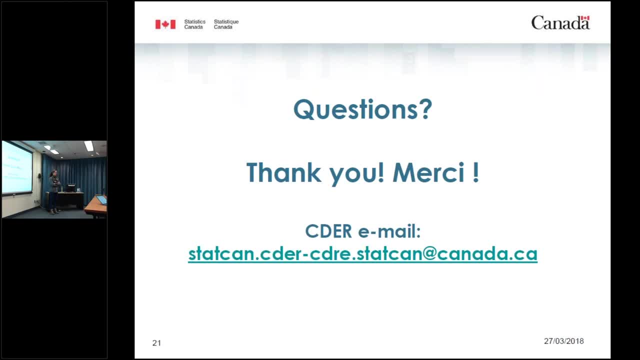 will be releasing a call for funds in the next two weeks for those of you who may be interested in applying. So now a question here by Benoit Dosti, Just wondering if you want to use T2Leap in the RDC network. 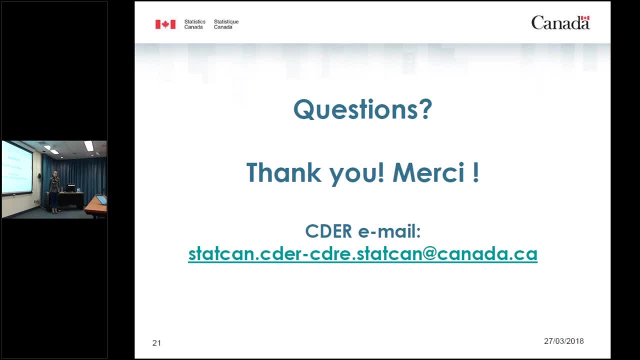 do you have to sign an asset disclosure agreement? Is it the same rule as in? Yes, yes, The same rule applies if somebody is working in the RDC as in CEDAR. OK, So it really the rules in terms of conflict. 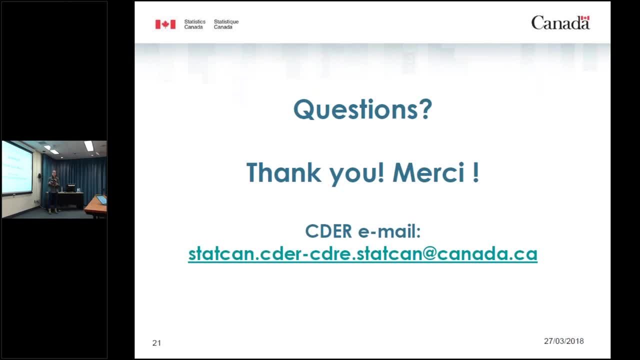 of interest and different asset disclosure requirements really are not based on the location of access, but more on what you are accessing, And so, with regards to access to business microdata, we want to ensure that no one has any conflict of interest when using the data. 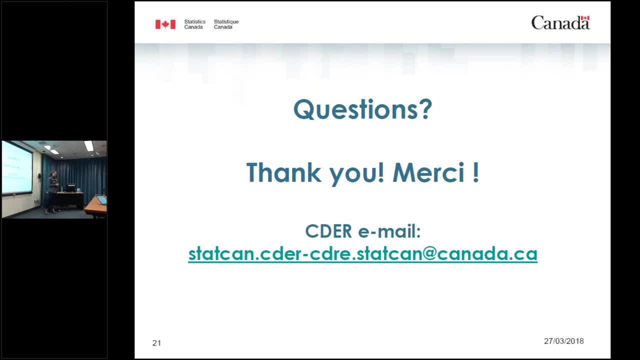 Thank you, And I'm starting to get some questions from people attending the webinar, So here's the first one, by Genthur Loma. I'm sorry, Genthur, I hope I'm pronouncing this correctly. So after the deadline of April 30th. 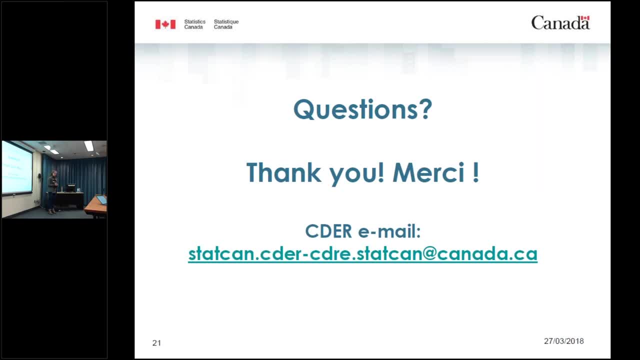 when will applicants hear back from the committee? And I have a follow up question: Will the data sets be officially available in the RDCs by summer 2018?? For the pilot purposes, yes, And so when are the project going to be approved? 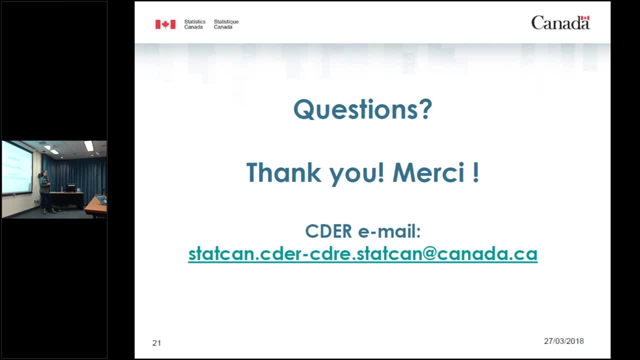 I can have a clear answer on that. And why is? because we're going to receive the proposal and we're going to do the evaluation. But if there's a proposal that really shows potential but maybe not be perfect, we might need sometimes to work with the researchers to help them maybe specify. 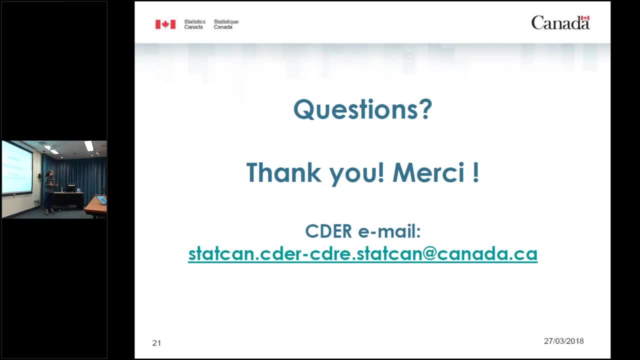 the proposal and modify it in a way so that it can be included in the pilot And the data, as we've mentioned, will be available in the summer, but really for the participants on the pilot only at this stage, But with the hopes that after the pilot. 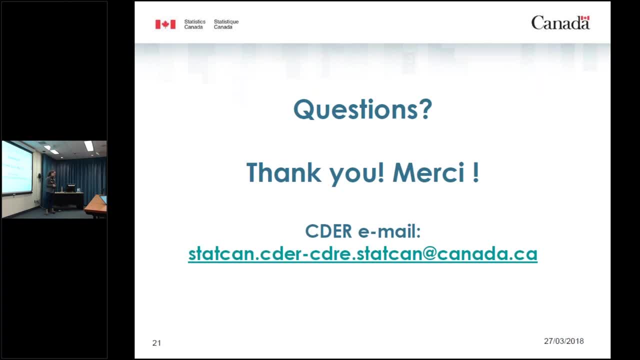 everybody can access it. Excellent, Thank you. And Here's a question by asking: can Leap be linked with any other data sets? Technically, yes, Leap can be linked with different data sets. However, for the purpose of the pilot, 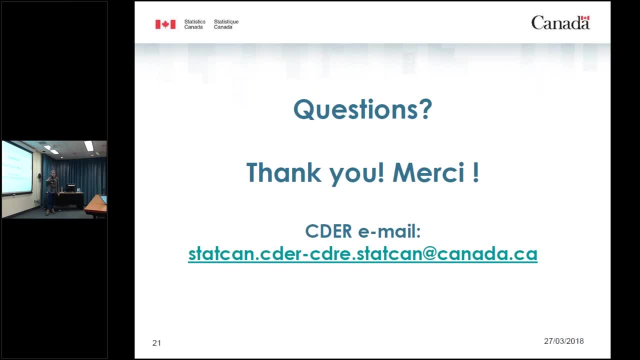 only this database would be available. If you're willing to look into using Leap with other database, I would suggest that you contact us at CEDAR directly and then we can discuss the use of different database. However, that would mean if you're using database that are not as 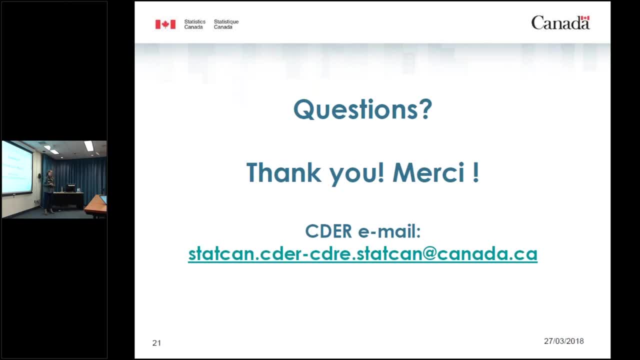 part of the pilot that the access would only be in Ottawa at StatsCan headquartered. Question by Andrea Craig. She's interested in estimating agglomeration externalities with these data. So two questions Here's: is firm location data available? first? 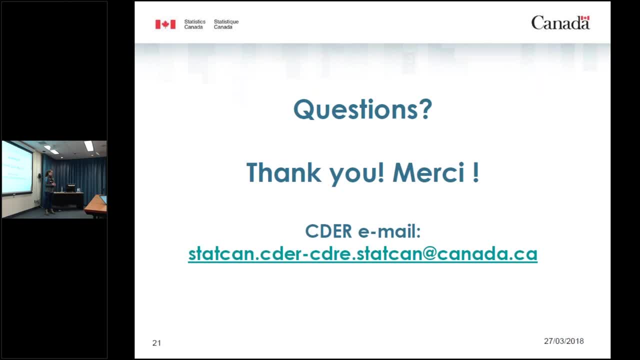 And then, if I restrict the analysis to small firms, would it be possible to get location data? Really depends on what you mean by location For the purpose of the pilot. the location that will be there will really be limited in terms of the detail. 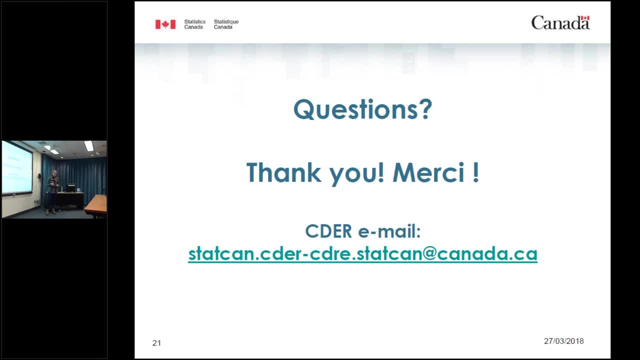 So for the purpose of the pilot, it might not be ideal. Also, one thing to remember, as I mentioned, is that Leap really is at the enterprise level, And so if you're looking at different agglomeration, for example by city or CMA, the problem. 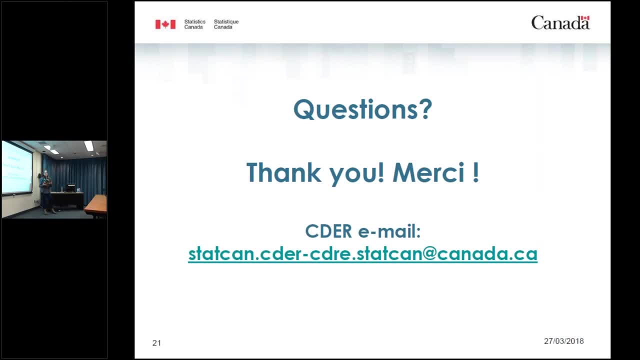 that you might encounter is that some companies that may be associated with one city or one province might actually have establishments all across Canada, And because the data is at the enterprise level, it means that, OK, That means that you will get a total employment. 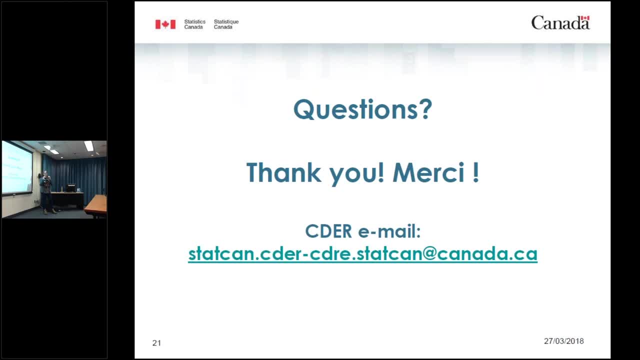 and total revenue that are associated with the whole enterprise, But that means that that revenue really is representative of the multiple location across Canada, which really could create some sort of bias and agglomeration studies. We have other databases, however, that can be used to do such research at CEDAR. 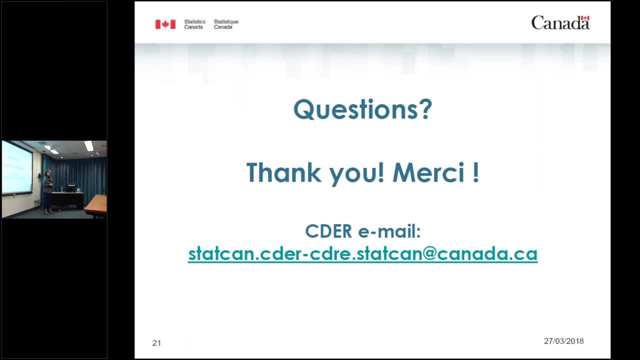 At the CEDAR. Yeah, But then it's outside of the pilot project. It's outside of the pilot project. They would have to pay for access, right, Mm-hmm. So eventually it would be available. Yeah. 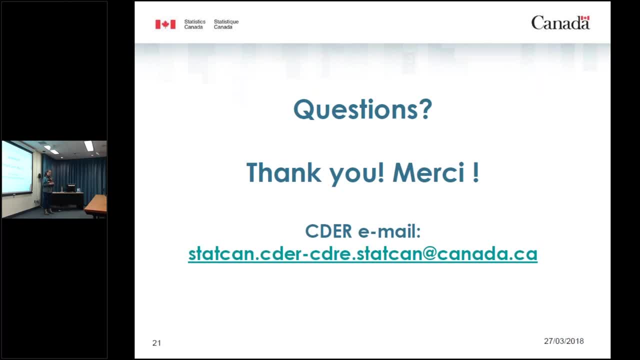 At some point in time. Well, we could discuss One thing that maybe could be done if the person- because the person is mostly interested for small firms, if we really limit ourselves to what we call a single, simple unit, so that are only present at the one location. 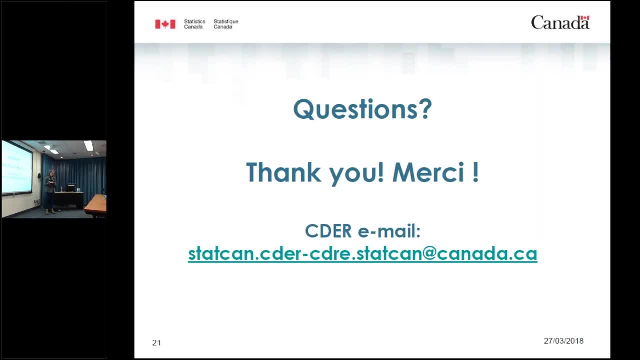 and are not across. that means that the enterprise level information really works with the one geographical location. What would happen, however, is that, for the purpose of pilot, the person would only have access to a very aggregated geography, maybe province at max. 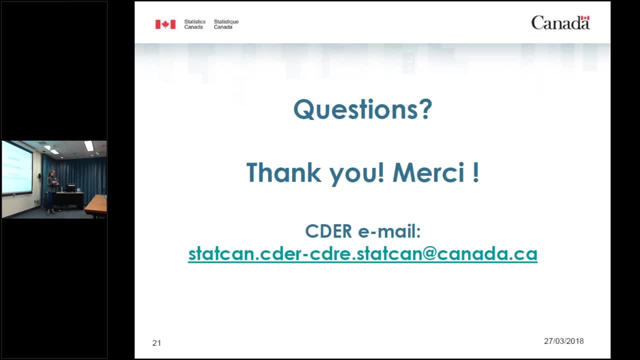 Mm-hmm For the pilot, For the pilot, But we might be able to run it. when we do a real, when we run the programs on the real data, we might be able to add extra geographical information and then do it. 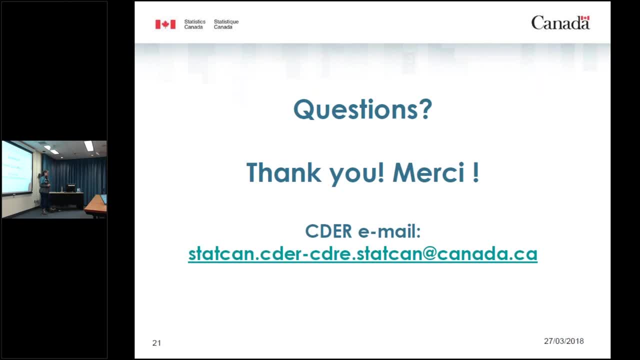 But we'd have to discuss that in more detail. Excellent, Thank you. Do you have any links to occupations of whoops? sorry, moved up. Do you have any links to occupation of these employees? No, at the moment we don't. 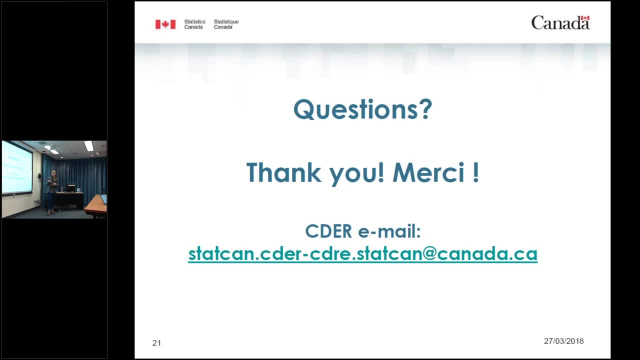 What one needs to really understand is that that database is enterprise level, So there's no information on the employees per se. It really is about the companies themselves. So you have the companies and you can see the number of employees that are in there, the total payroll that is paid. 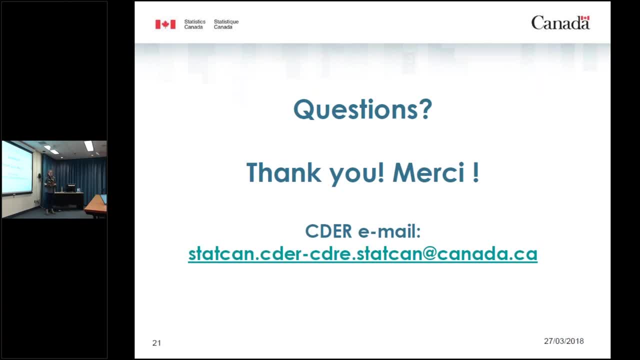 but you don't have information on specific employees. We have another database at CEDAR which is called the C, the Canadian Employer Employee Dynamics Database. It includes not only information on enterprises, but as well as information on individual employees. However, it does not include information on education. 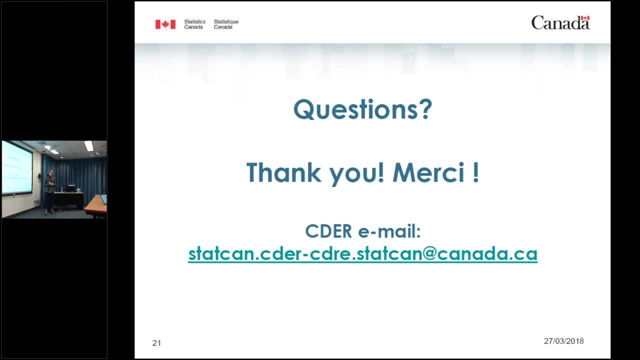 and occupation. yet That information will have to come from the census. There's a project to incorporate it, but it's for one or two years before we can use it. All right, Thank you. Question from Winter Lomas. A follow-up, I guess. 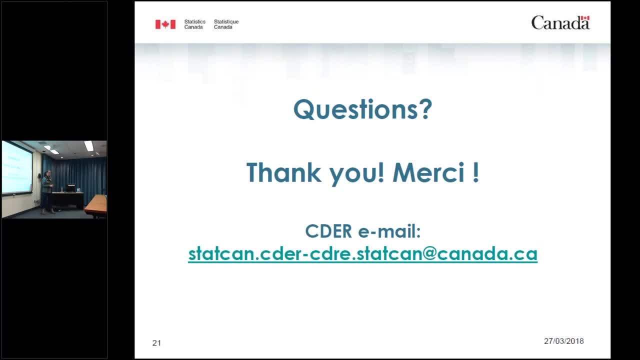 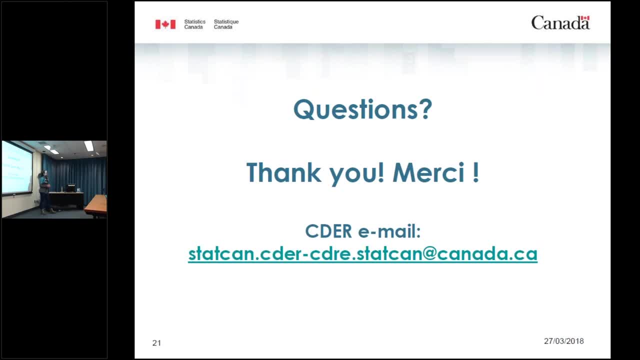 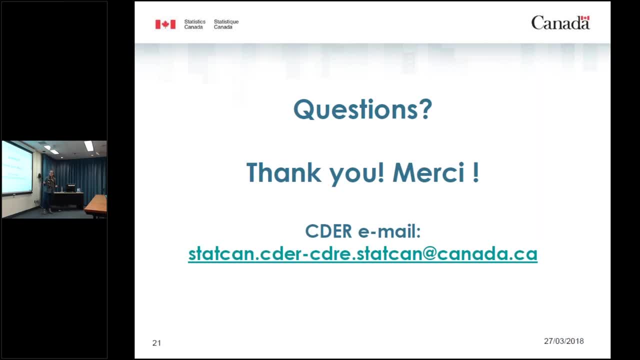 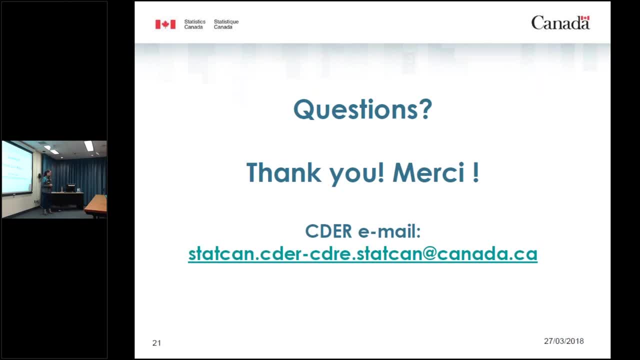 The synthetic data, or the data itself, really is based on administrative data. So T2Leap is created based on administrative data, So there's no question per se, but we do have a data dictionary that explains what the variables are, And the dictionary is available, right? 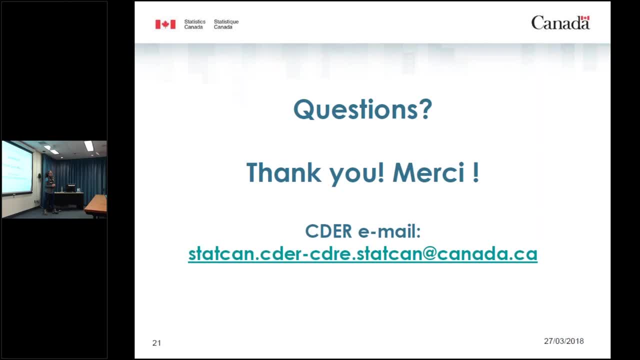 Yep Exactly, And he's continuing asking: does the test set include information on management practices? No, the data set really includes information coming from administrative data, So you can think, for example, when you file your taxes, that's the kind of information that we have. 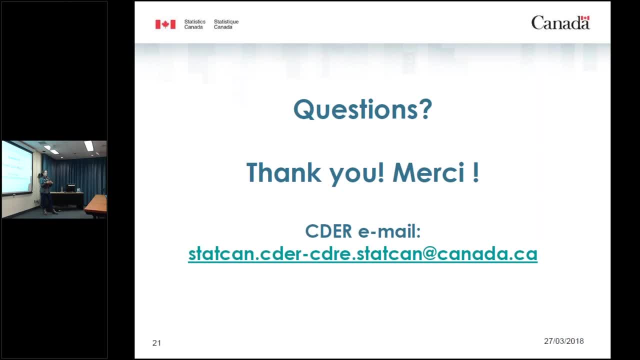 We have the information on number of employees and payroll based on the T4s like we fill when we do our taxes, And then we have the information that is required for enterprises to file when they do their own corporate taxes, which basically means that the variables that are included are variables such as the total revenue, total profits, assets and liabilities, for example, but nothing on management practices. 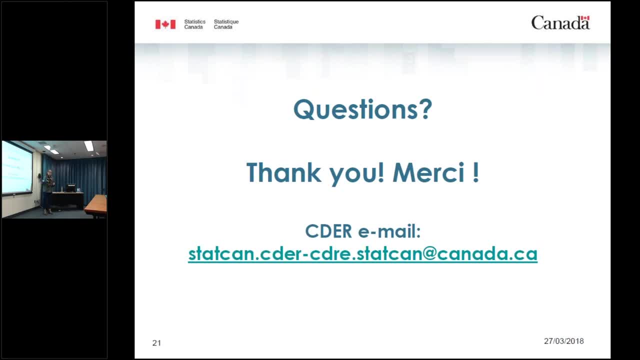 There are some surveys at StatCan looking at management services, for example the West Workplace Employee Survey. I believe It's an older survey that has been discontinued- The most recent year is 2006,- but it's still available for use at CEDAR. 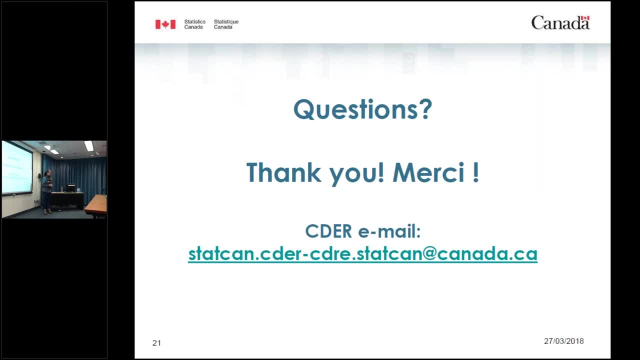 Thank you. I'm not sure I understand that one, but you are the expert. So do you have the number of firms and location within an enterprise? I guess he has several, So it is possible to identify the multi-establishment companies and the multi-province companies. 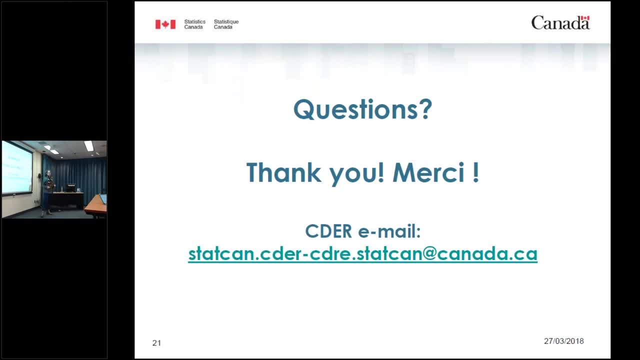 I don't think right now that we have a specific number of establishments per companies, but it's something that could be derived that we could discuss. Thank you, You said the call is for projects focusing on multivariate analysis. Does this mean output will be restricted to regression coefficients or would some of summary statistics be allowed? 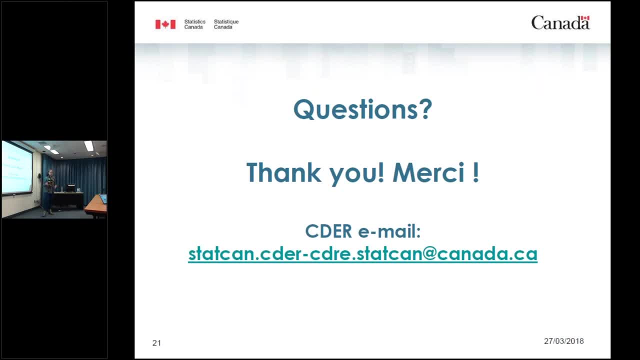 Some summary statistics can obviously be allowed. I mean, when we write papers and submit to journals there's always some summary statistics. but the summary statistics really has to support the analytical output and really must be limited. T2LIP is linked with other data set as well. 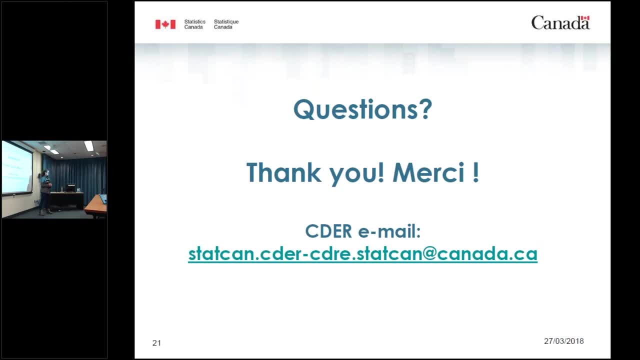 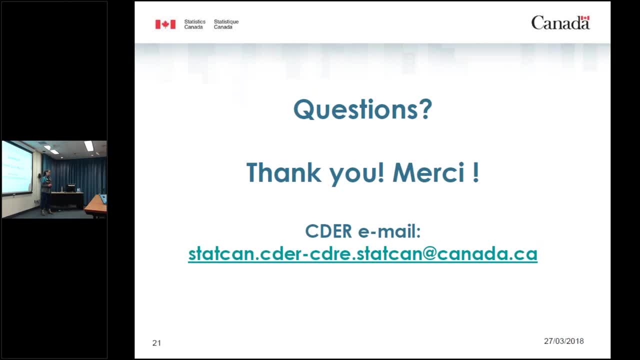 Not…. no, Okay, That's clear. Another one. Thank you all for your question. That's great. Alright, There's more of a comment here from Douglas May, But with T4 data you can determine the location of the employee using enterprise data, can you? 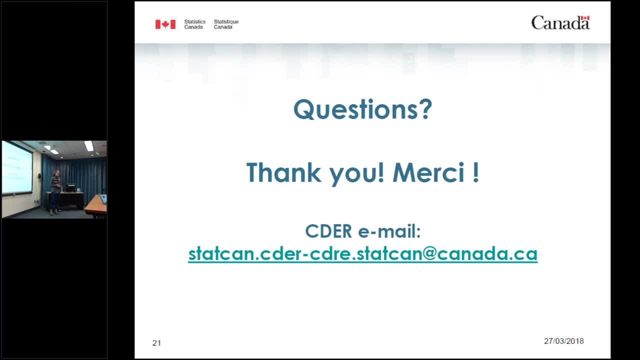 And identify interprovincial employees right. Technically, yes, we can do it. can do it, but not in this data set, because T2 Leap really is built to look at businesses. It's a database that is built to look at business performance, at business entry and exit. 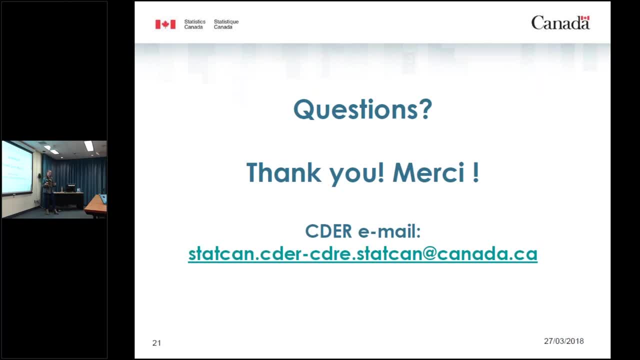 and this is what we start with the pilot, because it's a more simple database, It's more aggregated. We have other databases, though, that really use the detail of the T4, as well as the T1 and the T2, that combines both the information of the employees as well as the employers, but that's. 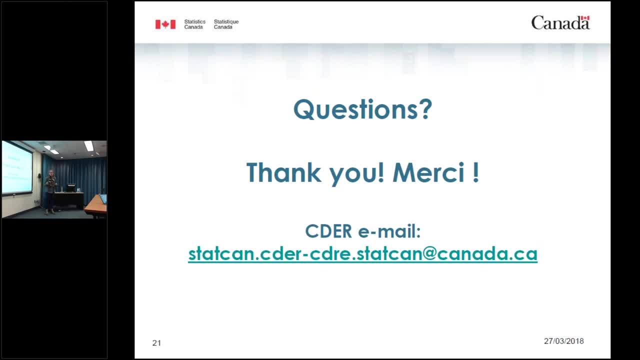 again another data set that we have. that's a lot more complex but it's very rich and it's available for use at CEDAR. It's the Canadian Employer Employee Dynamics Database. I have a comment from Yang Xingyi. He says that no sound at all. so I guess. 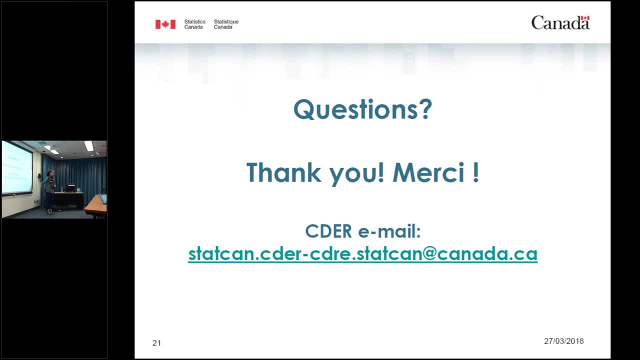 I don't know. Do you still have your? yes, I don't understand. It's 20 to 3. now, 3 minutes later, I hope you hear us guys. Anyway, I'm reading the question for sure. 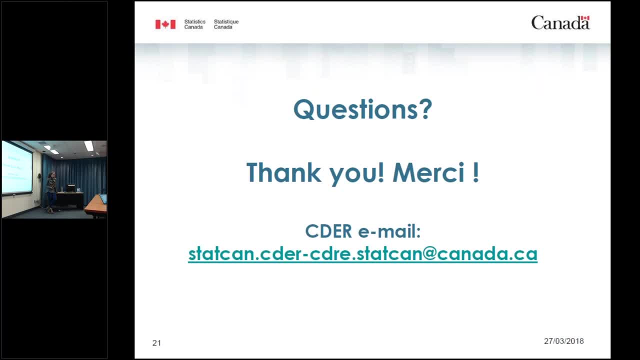 I have a question from Jeffrey X. I guess the people must hear us. because it's open, It should be functioning. So I have a question from Jeff: Are subsidiaries linked to parent companies? There is a way at StatScan, through the business register and through another division, that looks. 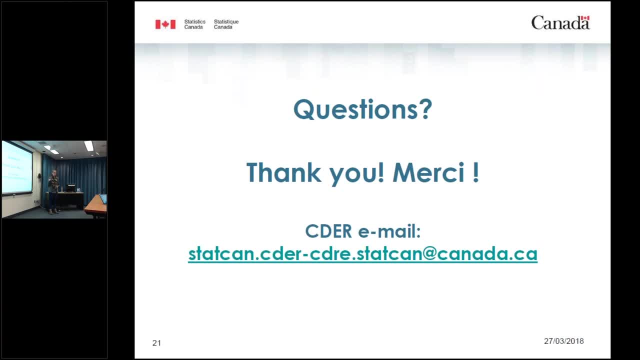 at the relationship between companies, to look at which businesses are part of which family of businesses, if you wish, In the T2 leap. however, it's really an enterprise-level data set and I don't believe that there is an indicator to see which ones are interrelated. 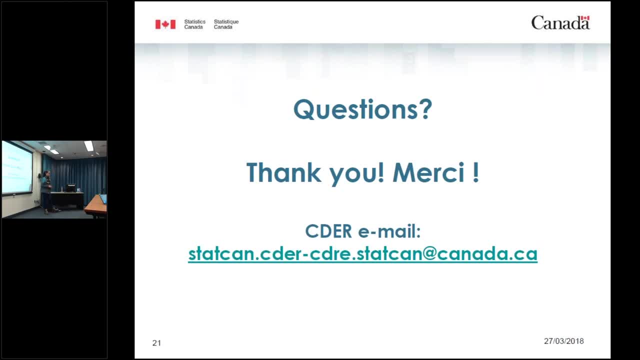 All right, Thank you. So that was the Last actual question. I will let a few moments still for people who may have last-minute questions. Many of you asked the question about whether the slides and PowerPoints would be available afterwards. 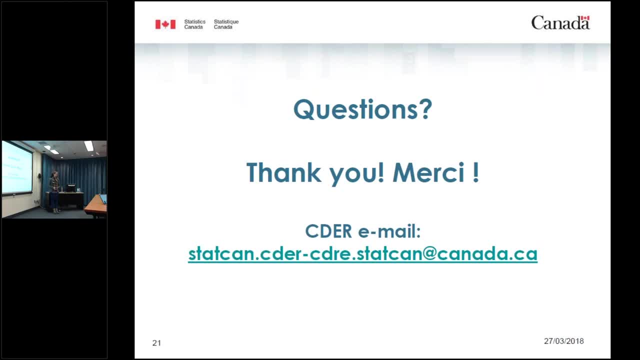 Yes, it will be. It will be posted on our website and actually the video, the audio video, will also be available on our YouTube channel. So that's it for now. Let me Close this. It seems to have a message somewhere. 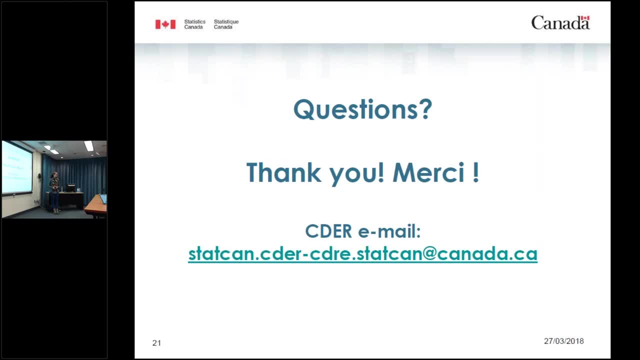 So that seems to be No. I'm sorry, I have another one here, Sorry, Yes, there's another question. Yeah, What is the time? coverage of the data? The data for the pilot is from 2001 to 2015.. 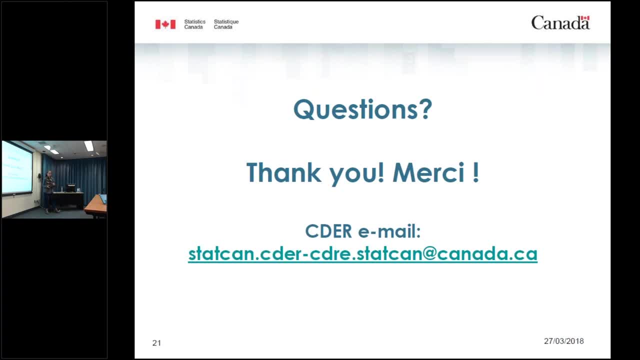 Excellent, Okay, Thank you. So it's 14,, 15 years, Okay, So well, I'm going to take a moment just to thank you, Lydia. If someone wants to write a question, I will take it afterwards. I'm just going to take the opportunity to 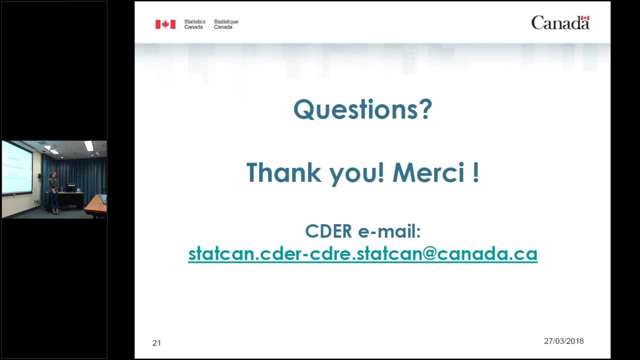 again, thank you for being here joining us. I wanted to say that our next webinar will be on April 23.. We will be discussing the impact of green spaces on people's health in urban areas. I also wanted to mention that we will be hosting the Networks annual conference.